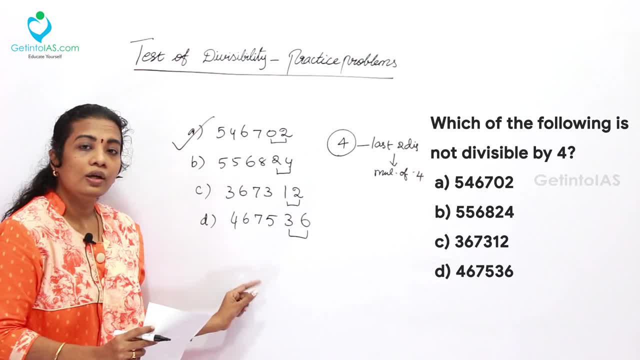 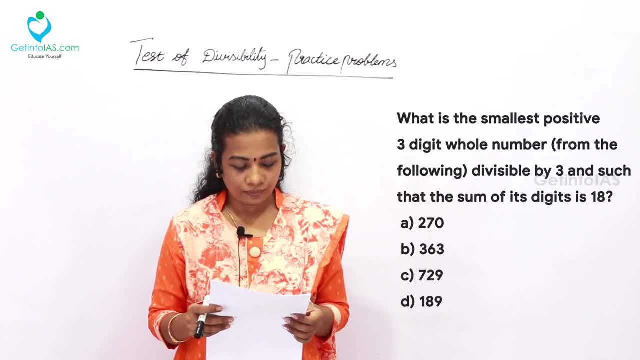 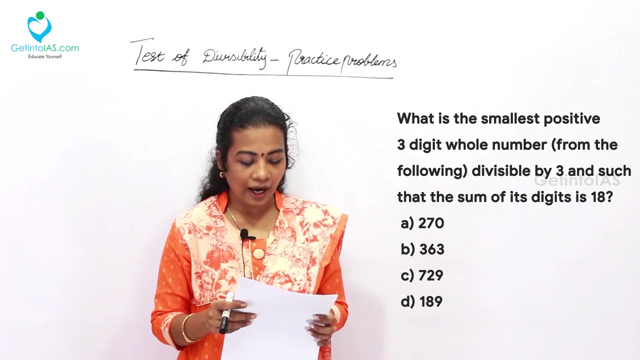 36.. 9 into 4 is 36.. So these all the three are exactly divisible by 4 except A. So answer for this question is option A. The next question: what is the smallest number of digits? So the answer is positive: 3 digit whole number from the following divisible by 3 and such that then, sum of its. 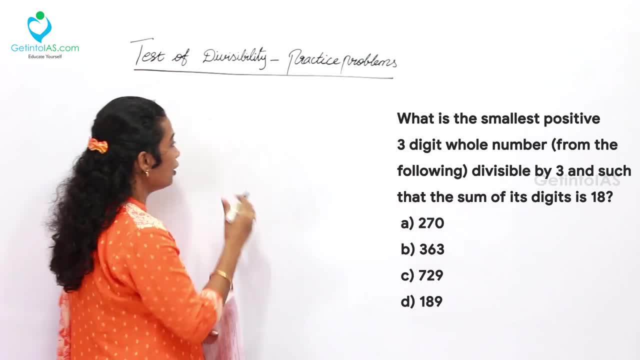 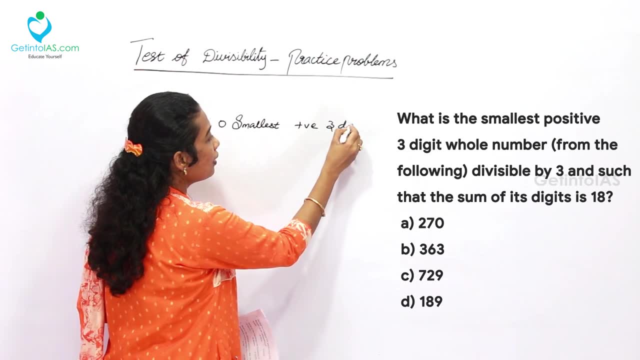 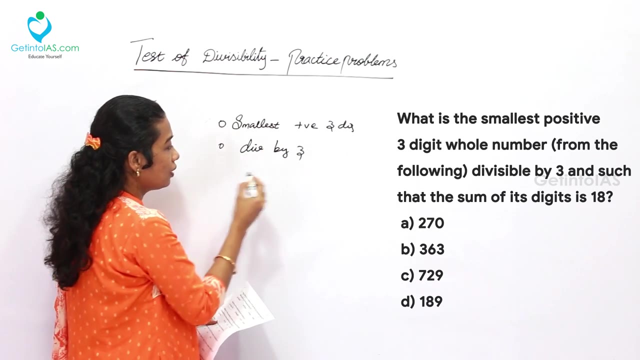 digits is 18.. Here three conditions are given in the question. The first condition is it is a smallest positive 3 digit number. The second condition says: which is divisible by 3.. Then the next one is: the sum of the digits is 18.. 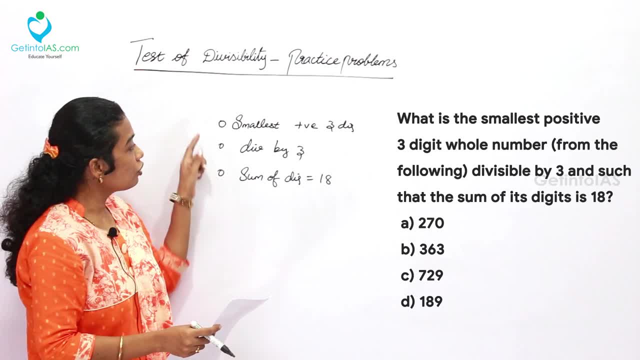 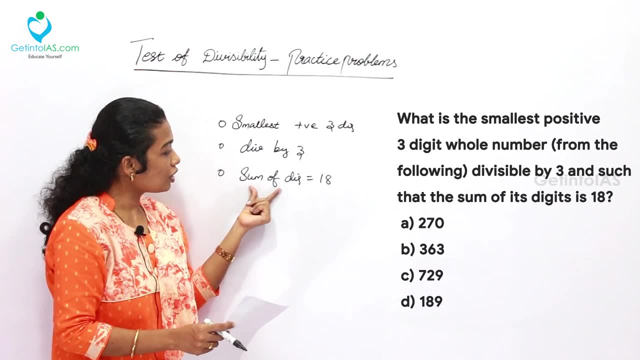 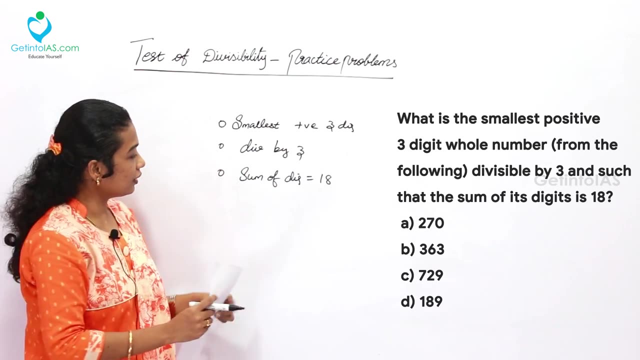 So that number from these options should satisfy all the three conditions. So, looking at the second and third condition, we know that sum of any digit which is a multiple of 3, then that number will be divisible by 3.. So, looking at the third condition, we can simply say no need to separately check for. 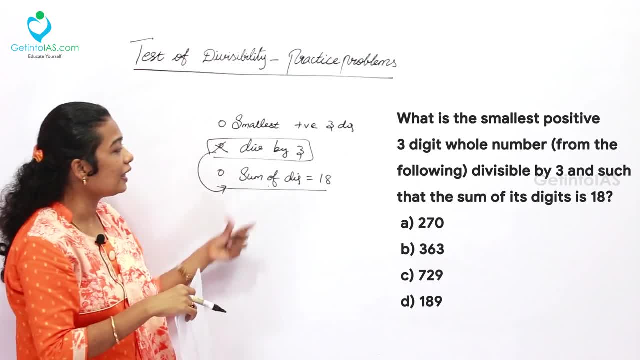 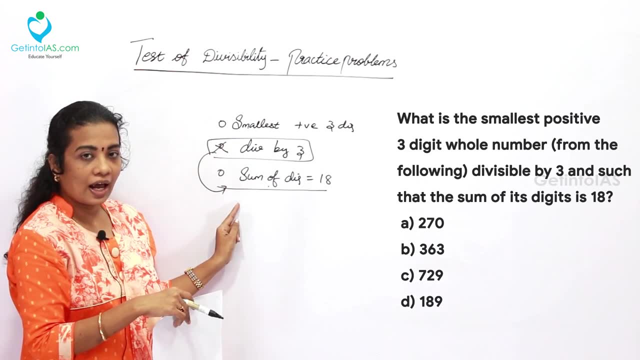 the second condition because the second condition automatically included in the third condition. So what we can do is, in order to check for the second condition, we can say the second condition only. we can go through these two conditions and we can check with the options one by one. 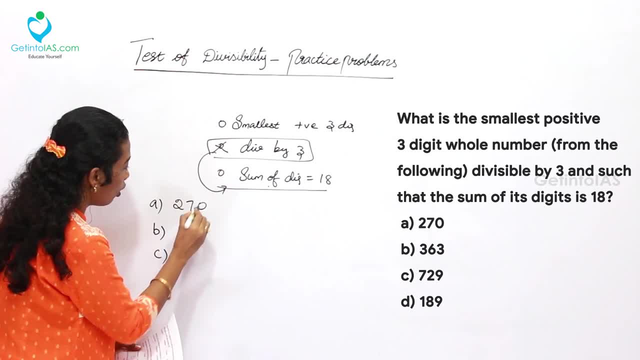 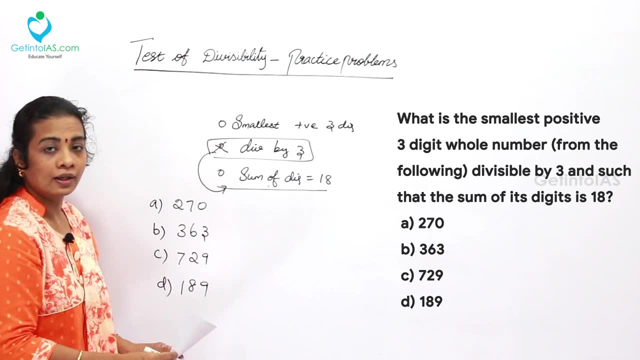 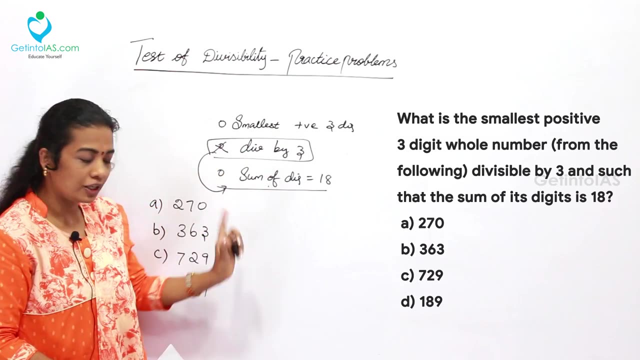 So option A 270, option B 363, option C 729 and option D 189.. Here we are going to check each of the options with the following condition: Smallest positive 3 digit number which is the smallest. here we can say D is the smallest number among the following conditions. So here we can say D is the. 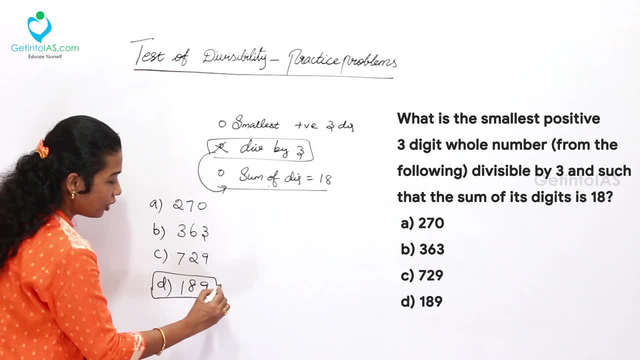 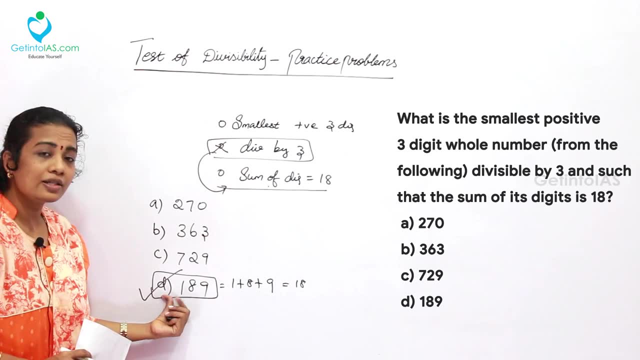 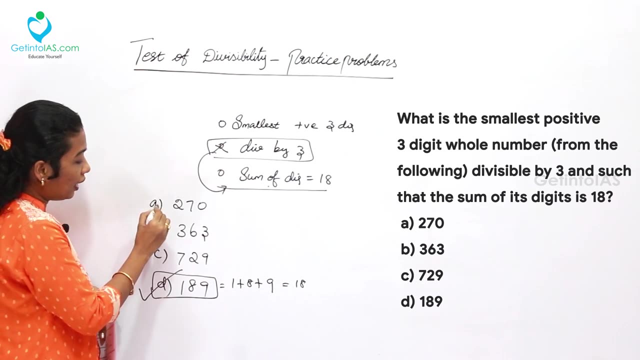 smallest number among the following: Okay, sum of the digits must be 18.. So here I am checking: 1 plus 8 plus 9, which is simply 18.. So I can easily choose. D is the correct option. Also, if you are, if you want to check for the other options, check A. A is not being the least number among the 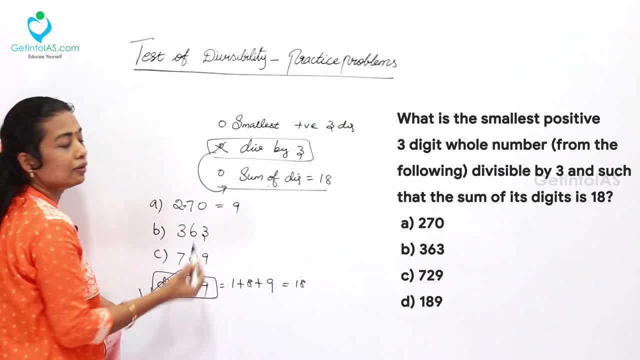 following: However, the sum of 2 plus 7 is going to be 9, which is against the conditions. So option A ruled out Option B: 3 plus 6 plus 3, which is going to be the smallest number among the following: 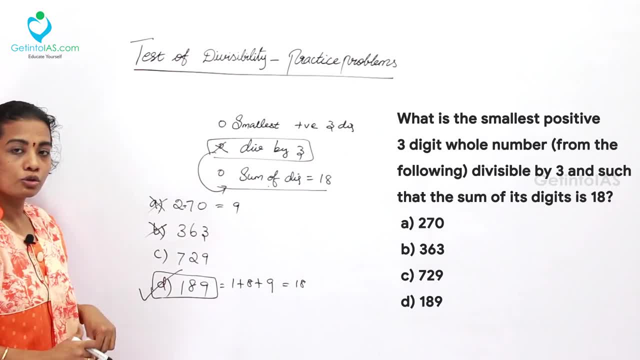 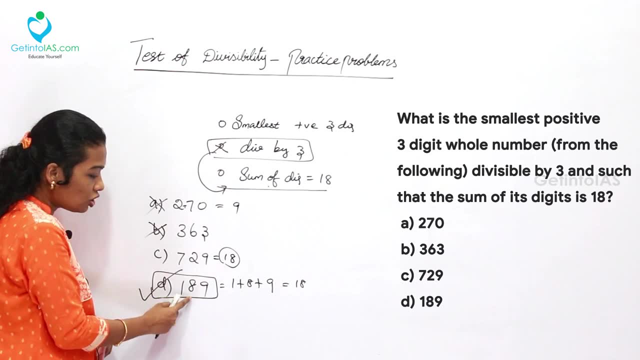 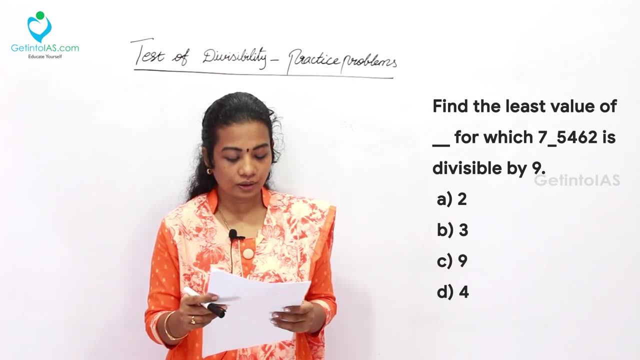 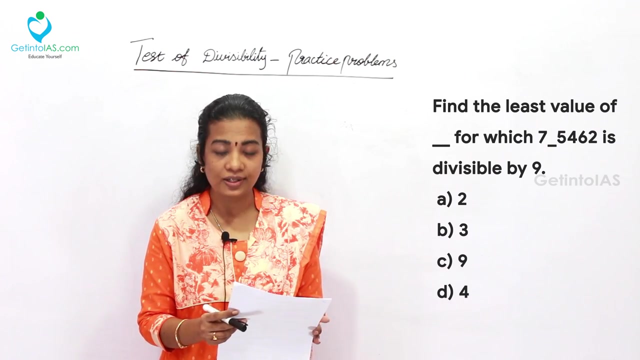 So option B is also ruled out. Option C: 7 plus 2 plus 9, which is 18.. However, among these two numbers, which is the least one? option D, So option C is also ruled out. Finally, the answer is option D. The next question: find the least value of underscore, for which 7 underscore, 5, 4, 6, 2 is. 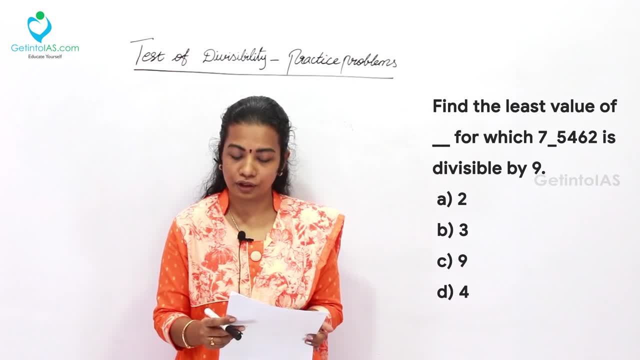 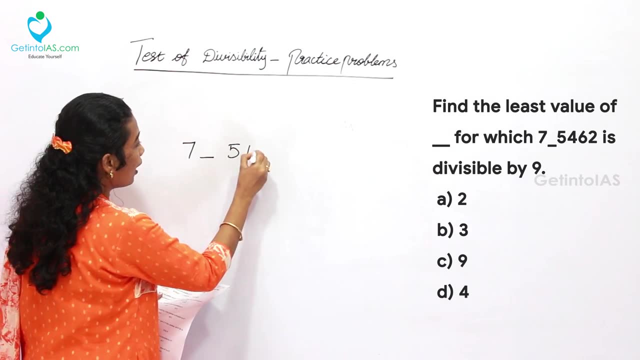 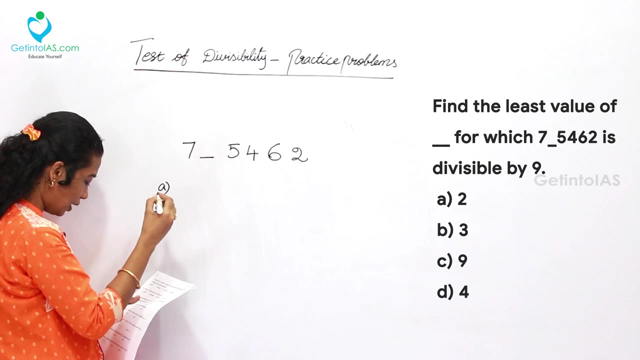 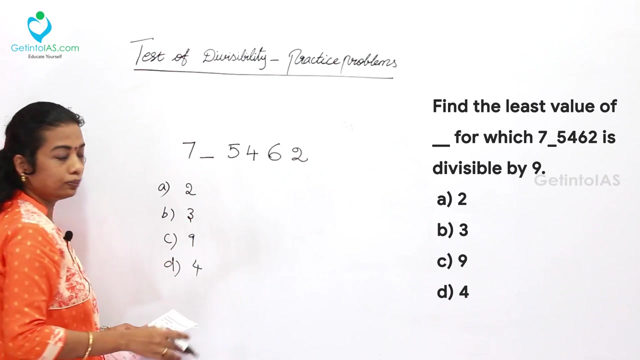 divisible by 9.. So here, four options are given in front of you. The hidden trial method. The given number is 7, dash 5, 4, 6, 2. You will have to find the number. What is the number to be placed over here? Your options are A, 2, B, 3, C, 9 and D, which is 4.. So let's 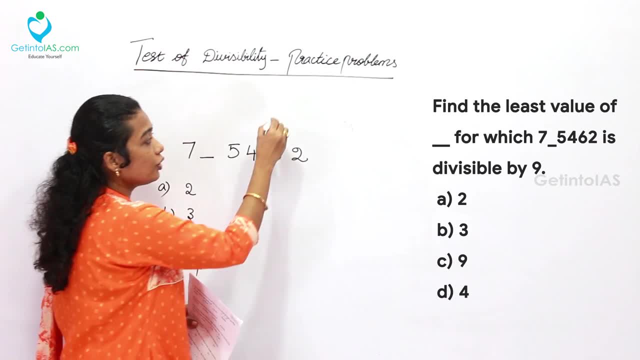 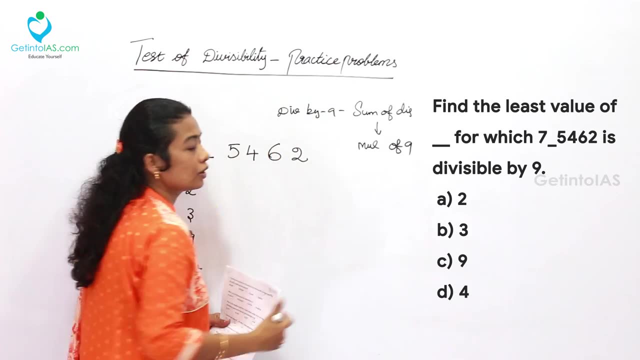 take it This number should be divisible by 9.. What is the rule for divisibility of 9.? The sum of digits should be divisible, So the sum of the digits should be a multiple of 9.. Let us check 1 by 1.. Here option A, which is given: 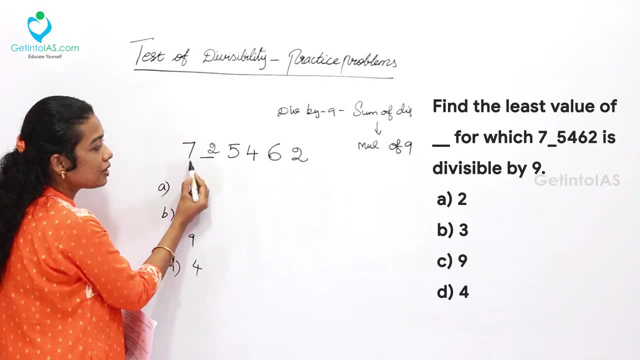 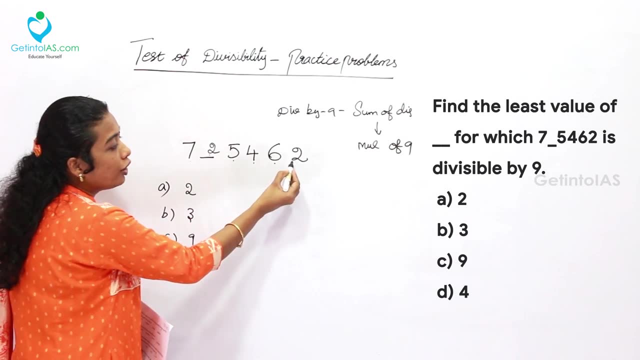 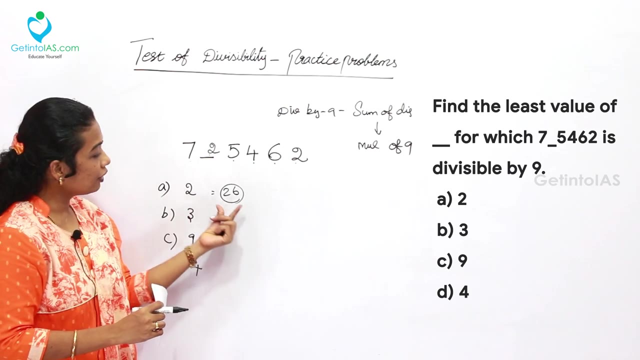 2. Let me take 2 over here. Now you can add up 7 plus 2, 9. 9 plus 5, 14. 14 plus 4, 18. 18 plus 6, 24. 24 plus 2, 26. If I would have been taken this 2 over here, the final result will be 26, which is not. 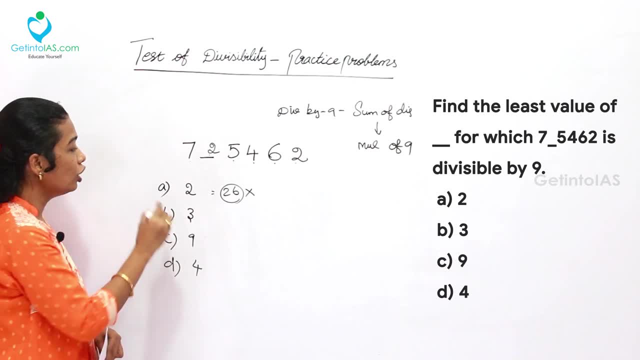 a multiple of 9, because 9 into 3, which is 27. so option a ruled out. let us take option b, 3. let us make 3 over. here. i have accommodated 3. now you can simply add all the digits, so or you can just include 1, 26 already. 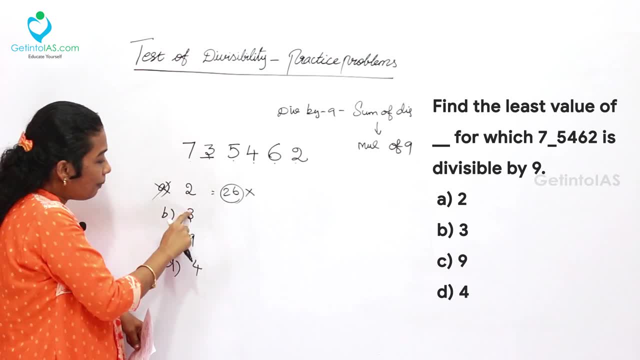 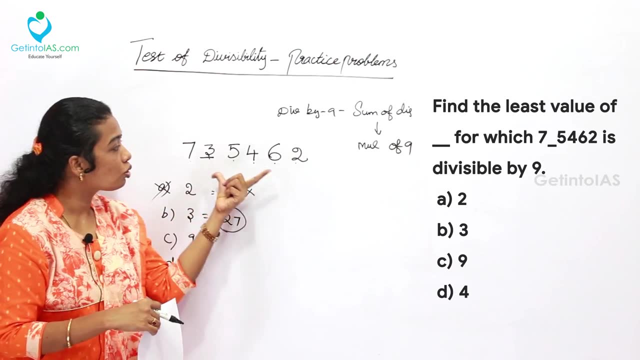 we had, with the help of accommodating 2 over here, plus 1 we have increased right, so definitely it is going to be 27. 27 is a multiple of 9, so this number- 7, 3, 5, 4, 6, 2- is going to be the. 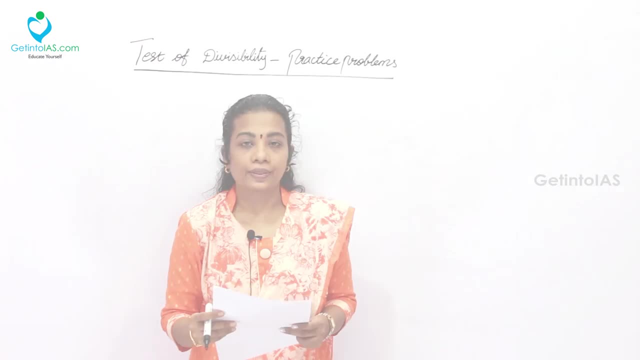 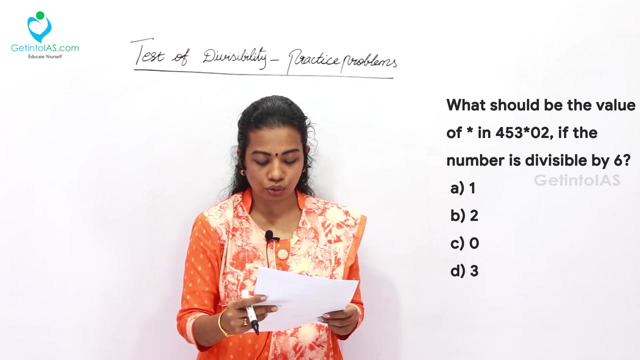 multiple of 9. so option b is the correct one. the next question: what should be the value of star in 4, 5, 3, star 0, 2 if the number is divisible by 6? here also, 4 options are given in front of you. 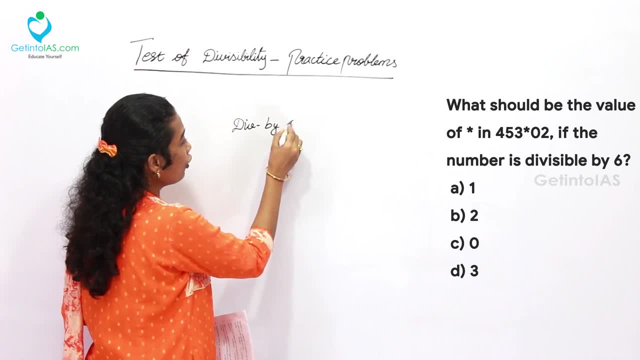 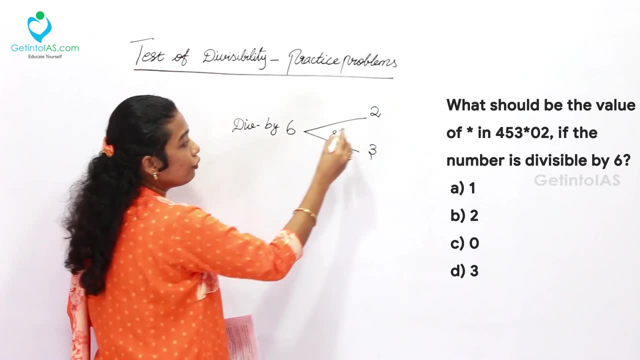 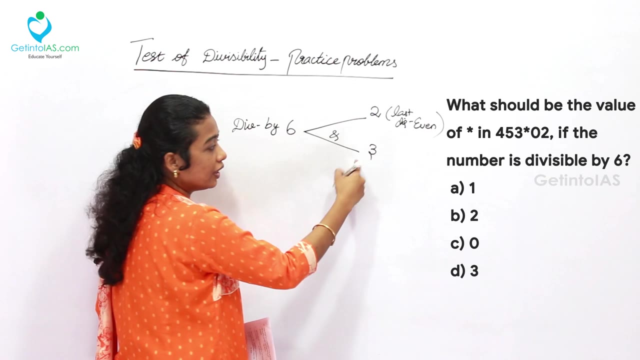 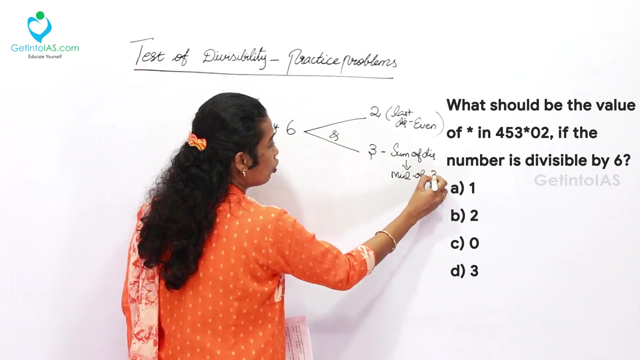 so what is the divisible by 6 rule? that number should be divisible by both 2 and 3. what is the rule for 2? the last digit should be even. and what is the rule for 3? some of the digit should be multiple of 3, so which number? 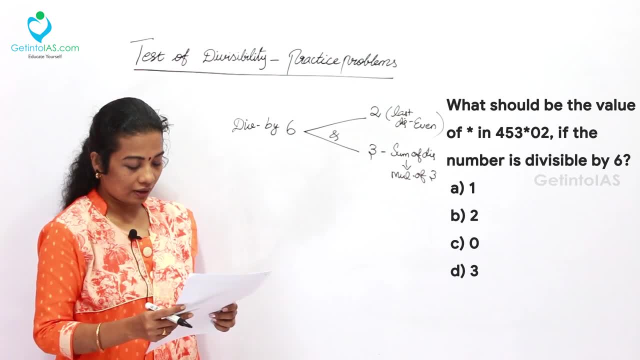 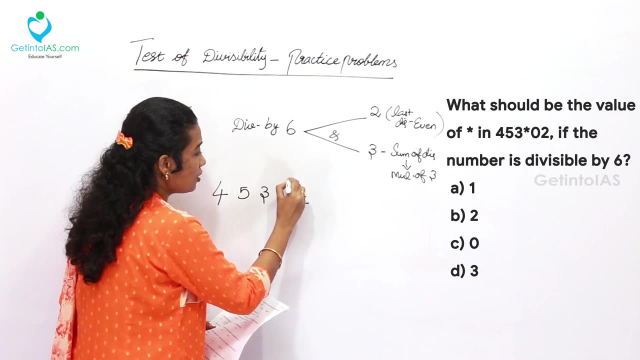 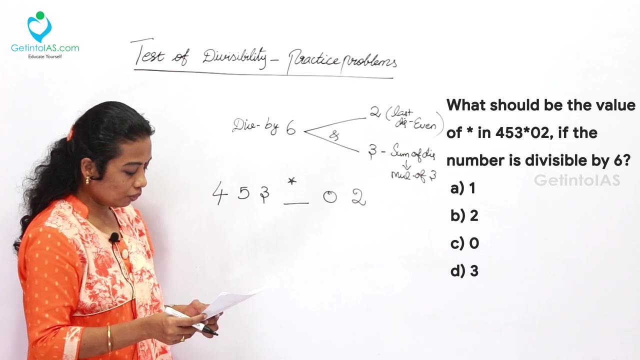 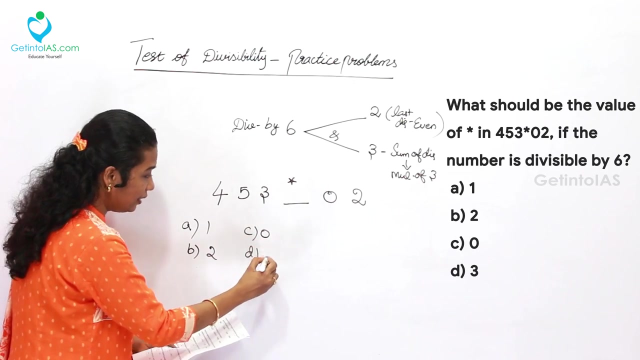 is satisfying these two condition will be the correct answer. what is the number given? here is 4, 5, 3, here it is star, 0, 2. somewhat number is going to be placed over here. so, looking at the option, we are having a, 1, b, 2, c, 0 and d. we got 3. so first i am taking the 1 option, 1 i am. 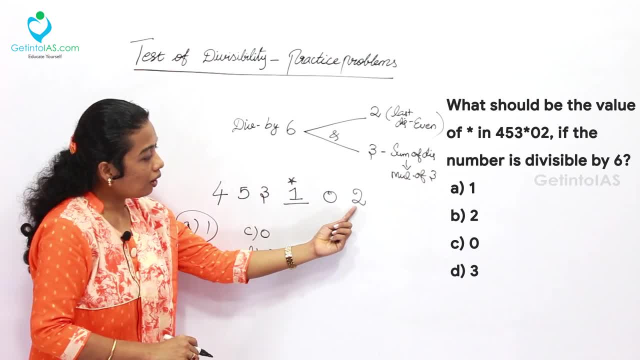 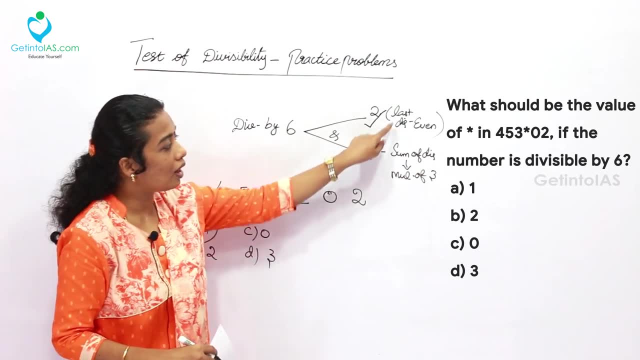 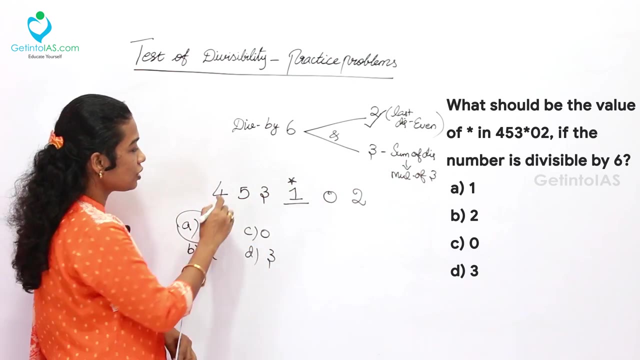 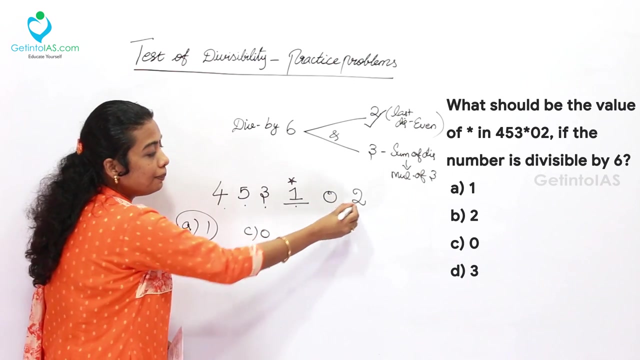 placing 1 over here. now you can check already. 2 is here, so definitely this number is going to be divisible by 2, why? because the last digit is even already. then the next condition: 3. some of the digit should be the multiple of 3. simply, you can add up 4 plus 5, 9, 9 plus 3, 12, 12 plus 1, 13, 13. 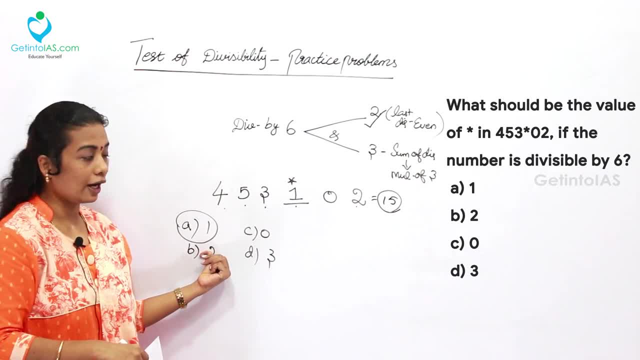 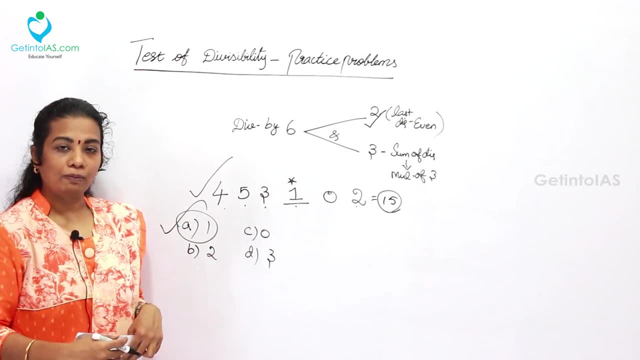 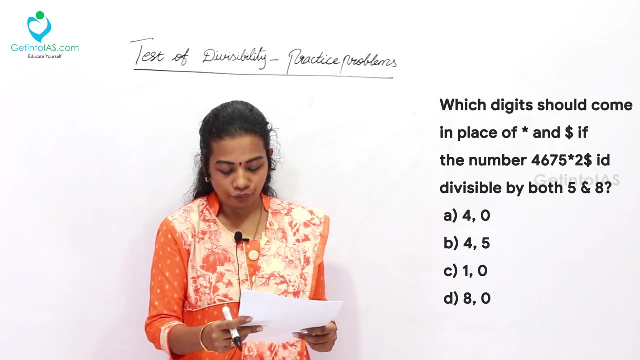 plus 2, 15. i got 15 as the result while applying option a, so 15 is being the multiple of 3. this number is also a multiple of 3, so option a is the correct one. the next question: which digit should come in place of star and the dollar symbol if the number four, six, seven and five star is positive? 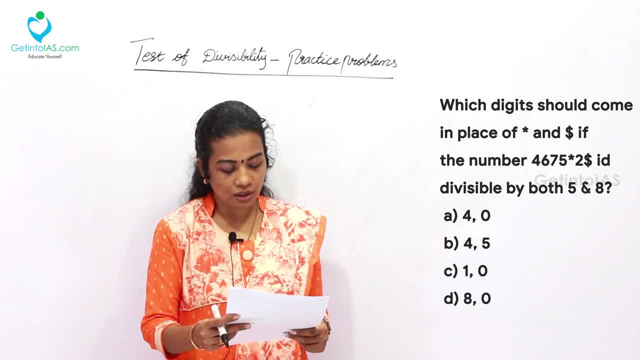 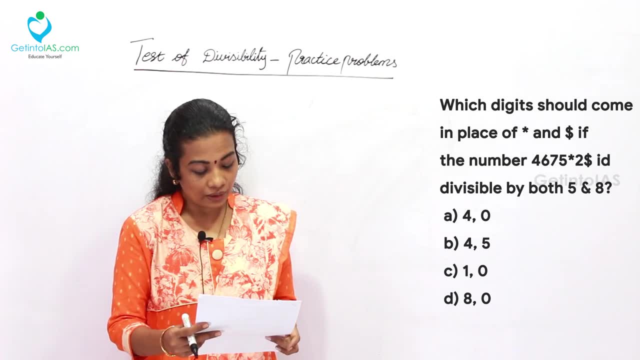 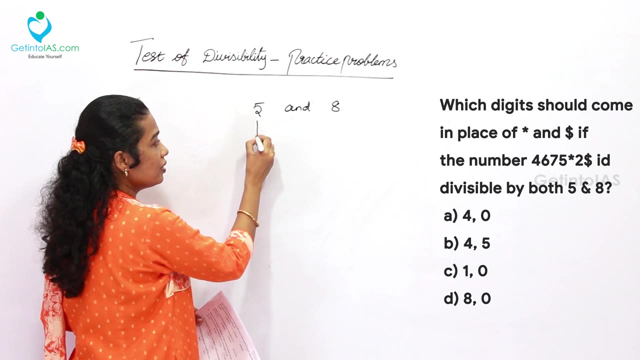 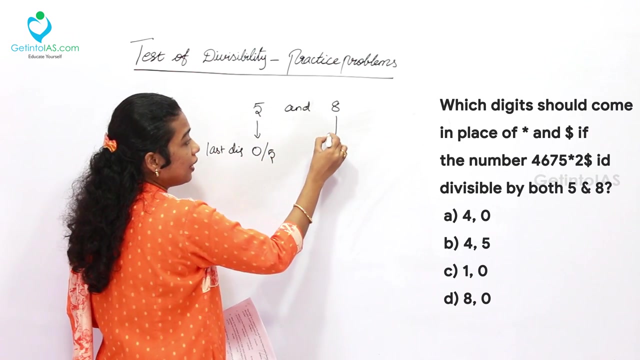 six, seven, five star two dollar is divisible by both five and eight. as of now, we have seen only one number divisibility rule here. we got two numbers combination, that is for five and eight. for that, what is the rule? for five, the last digit should be zero or five. what is for eight? 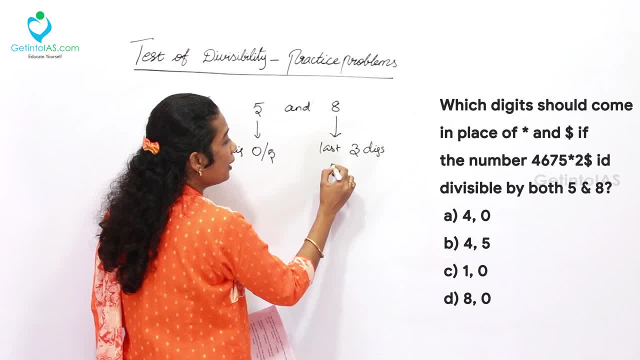 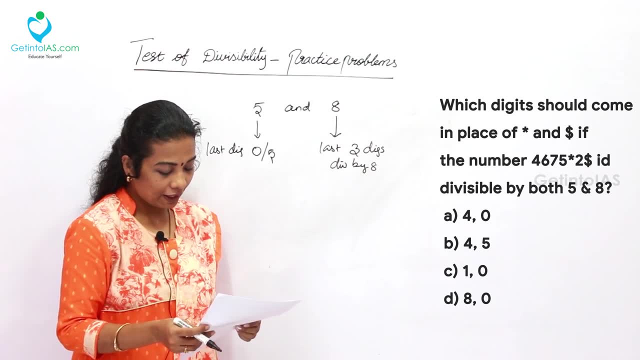 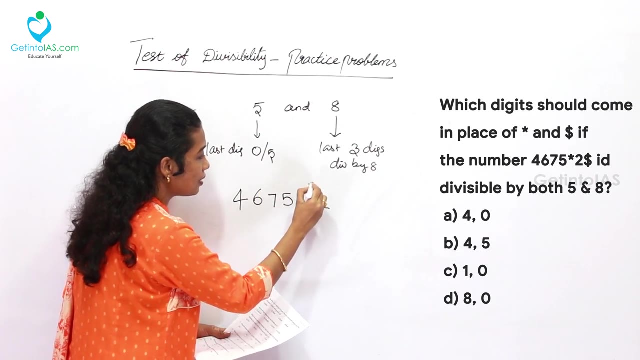 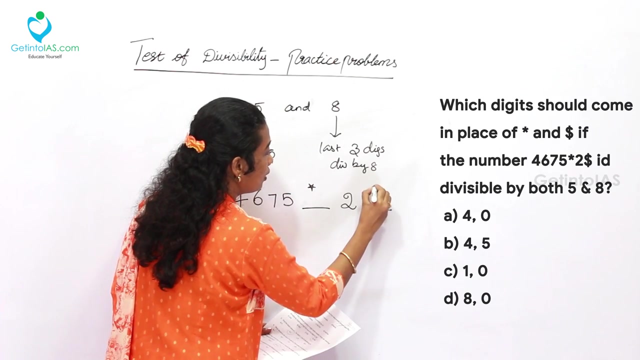 the last three digits should be divisible by eight, which means the last three digits should be a multiple of eight. so let me take the first thing, four, six, seven, five, and here star symbol is given, and after the two then dollar symbol. let me take, like this, the dollar symbol over here. 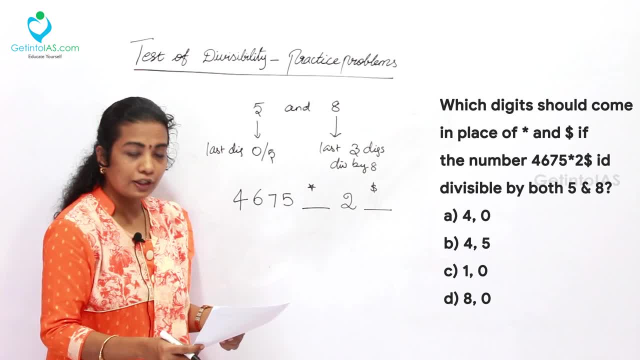 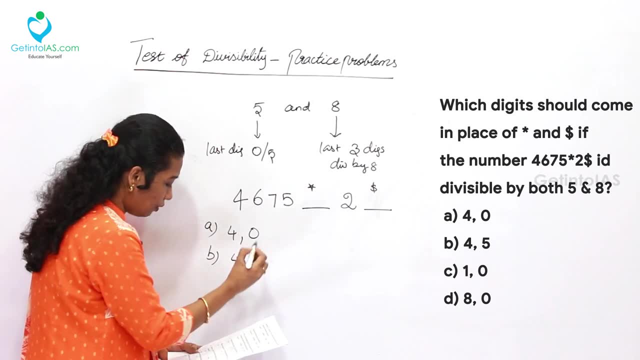 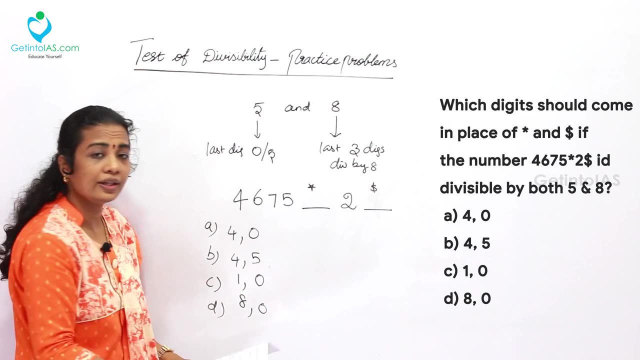 now, what are the numbers are to be placed over here here, set. the number of numbers are given in every option: option a: four and zero. option b: four and five. option c: one and zero. and option d: eight and zero. in these cases, no need to confuse in the first. 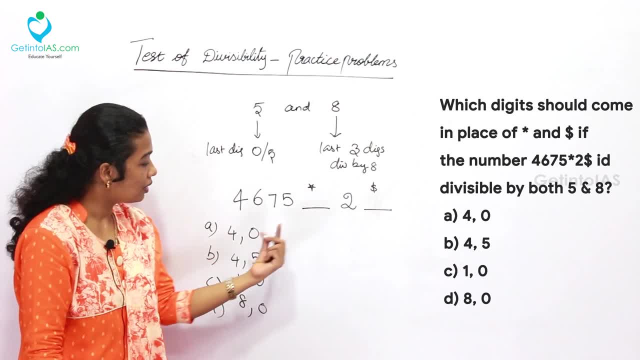 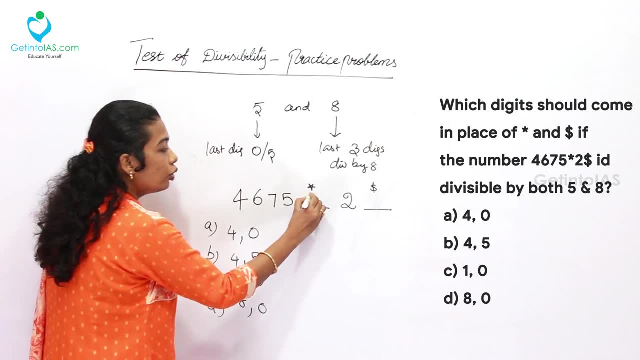 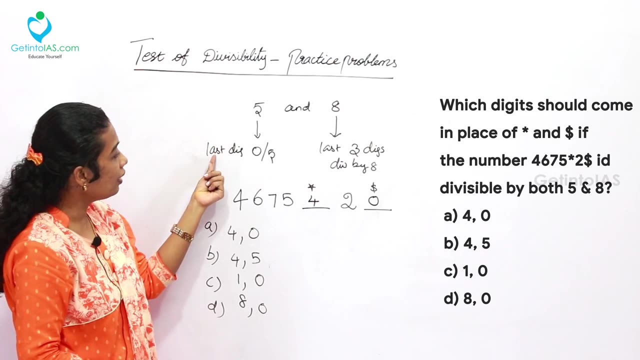 place, first number is to be accommodated. in the second place, the second digit is to be accommodated respectively. so let me check for the first one. let me take four over here and zero over here. now, checking with the tester of deciability of five. last digit should be zero or five. 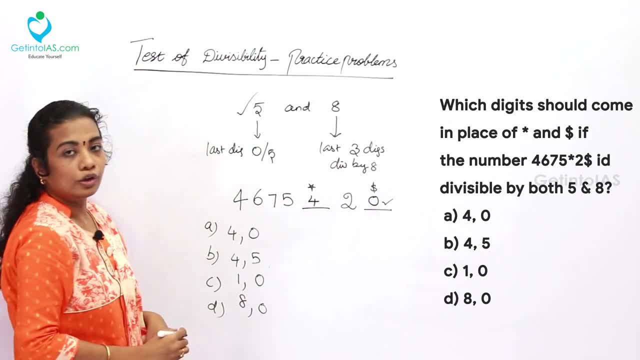 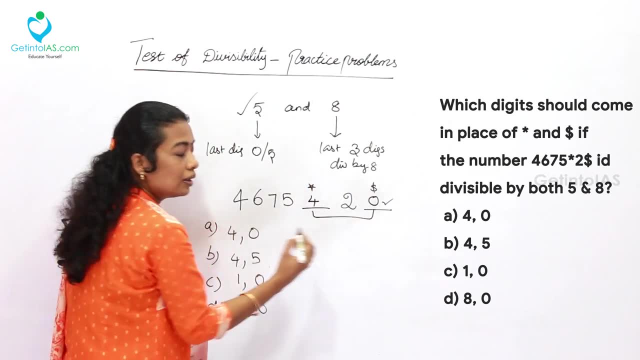 yes, satisfied, so I can put tick over here. and what about eight? you want to take? the last three digit should be a multiple of eight. let me check for. Twinties is the last three digit. so 420 divided by eight, so 4 times 8 is 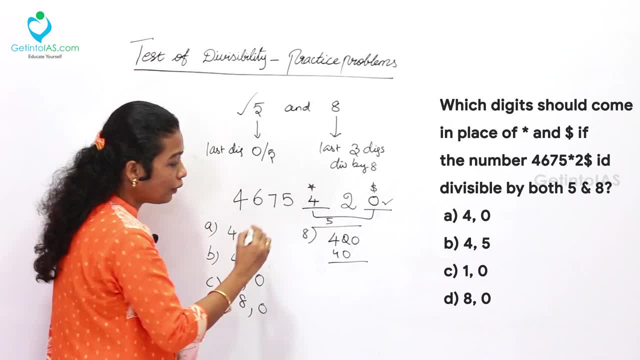 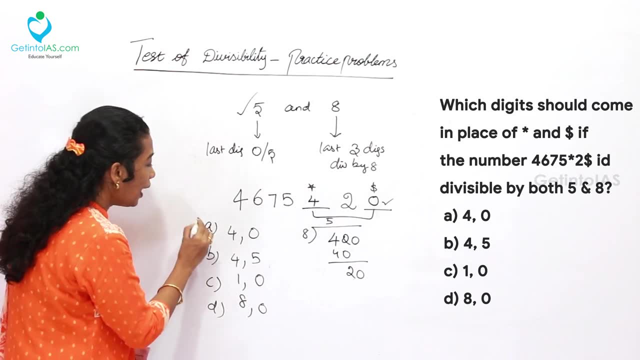 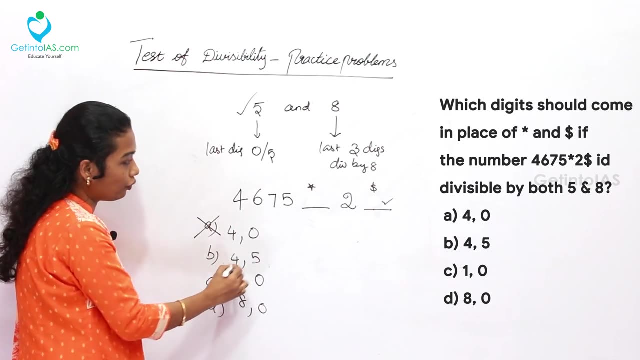 thirty two to five times 8 is 40.. Forty is a multiple of eight, then twenty. what about 20? 20 is not a multiple of 8, so we can eliminate option a. then, moving on to the second option, first place is to be filled with 4 and the next place is to be filled with 5. here, 4 and here. 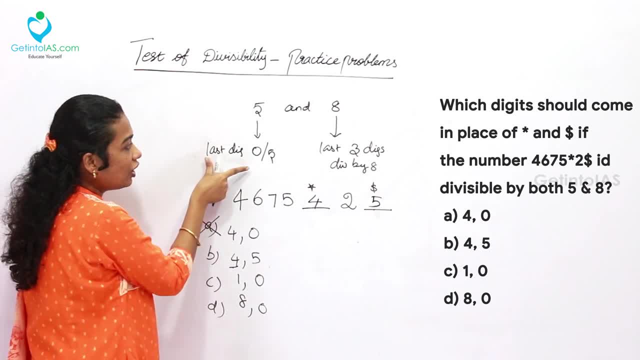 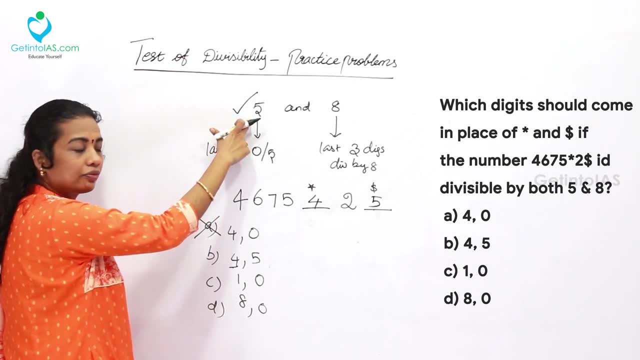 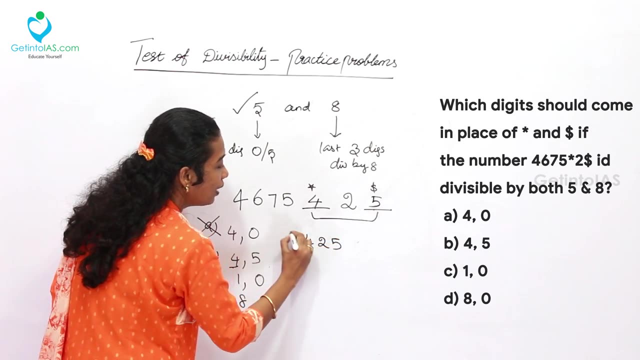 5. now let me check with the 5 divisibility. this last number is 5, so last digit 0 or 5? definitely this number is divisible with 5. then what about 8? you want to take the 3 numbers at the last, so 425. i am simply going to divide with 8. here the quotient part is not required, simply. 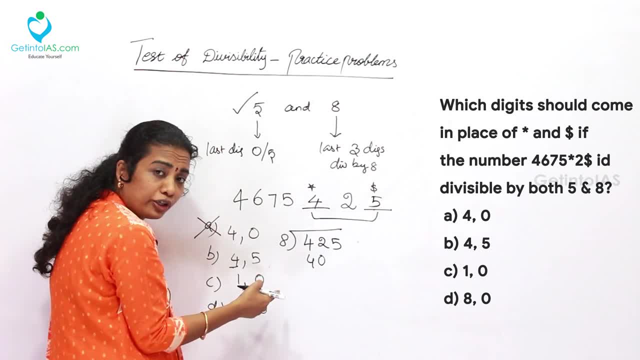 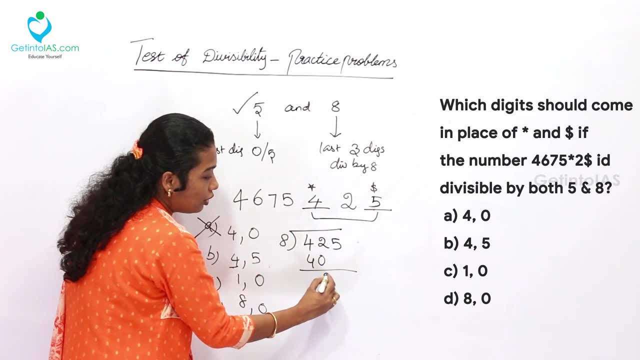 you can say 40. why? because only we are going to check with the divisibility rule. no need the quotient part. so 5 into 8 is 40. i am not going to write 5, so here: 25, 25. simply check whether 25 is. 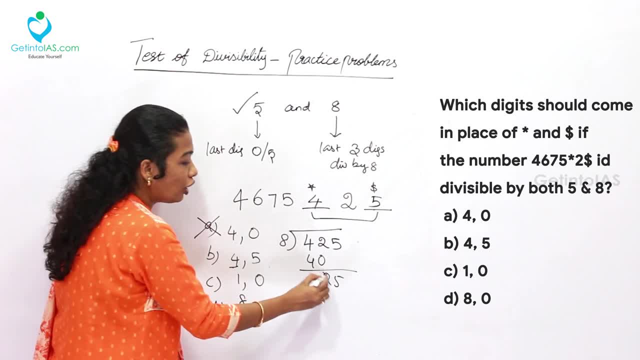 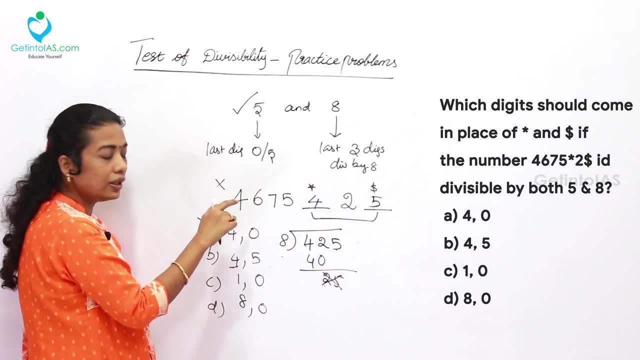 a multiple of 8 or not. no, 24 is the multiple of 8, not 25. so this 425 is a, not a multiple of 8. this whole number of 7 digit number is not going to be a multiple of 8. so simply option b ruled out. then the next one. 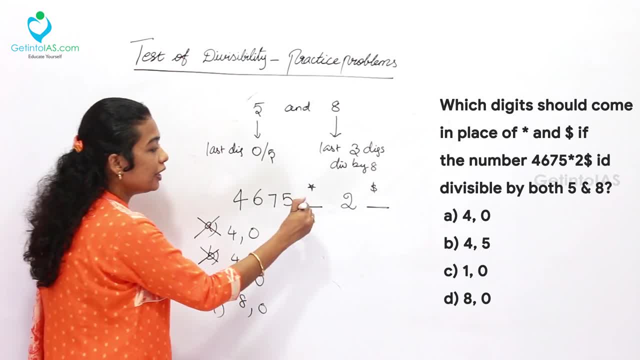 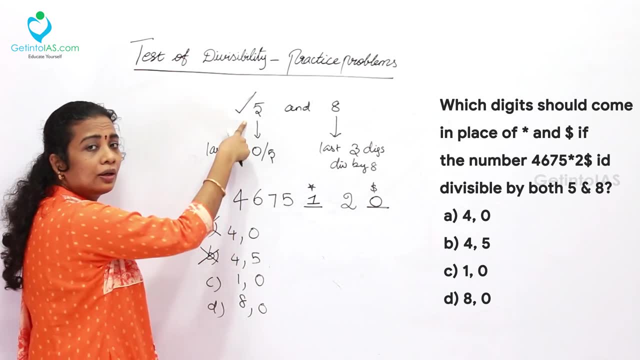 moving to the option c, 1 and 0. simply, i am going to accommodate 1 and 0 over here. as soon as i place 0, definitely this number will be multiple of 5. then what about the other things? i am going to take the 4 and the next one. i am going to take the 4 and the next one. 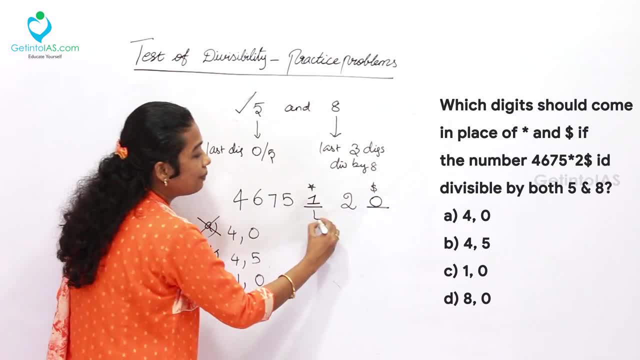 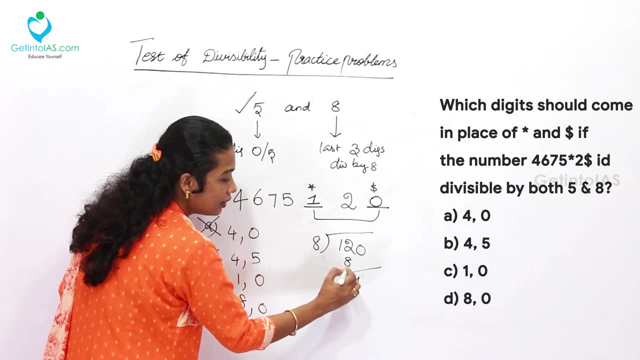 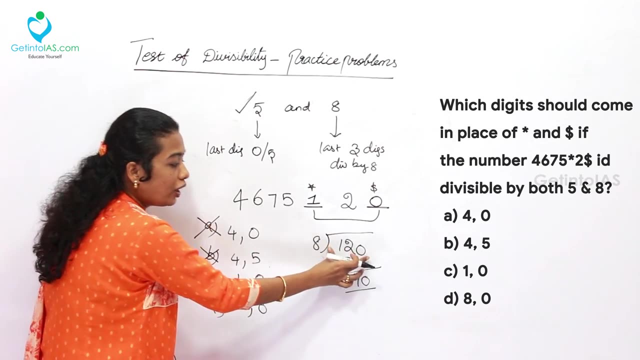 last three digit divisible by 8. so i am picking up the last three digits: 120. i am taking here 8, so 1 time 8 is 8, then 4, 40. 40 is a multiple of 8 by 5 times, so 40 is a multiple of 8, 120 is. 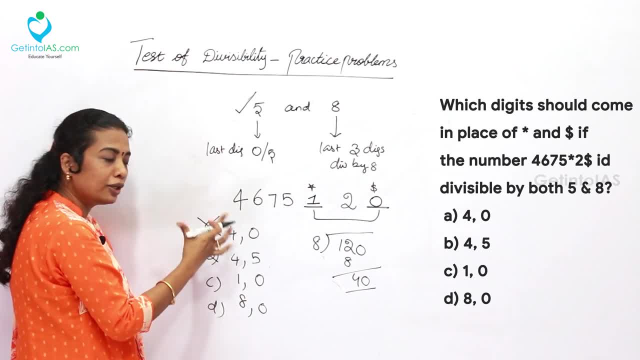 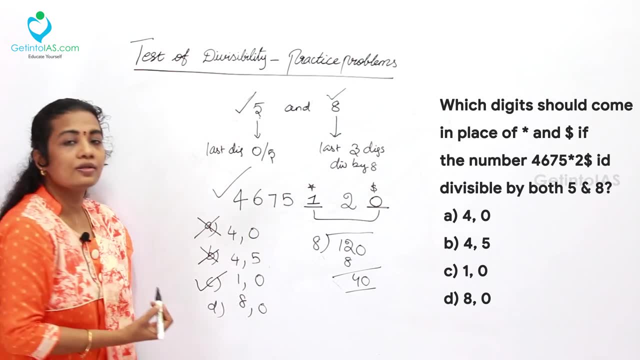 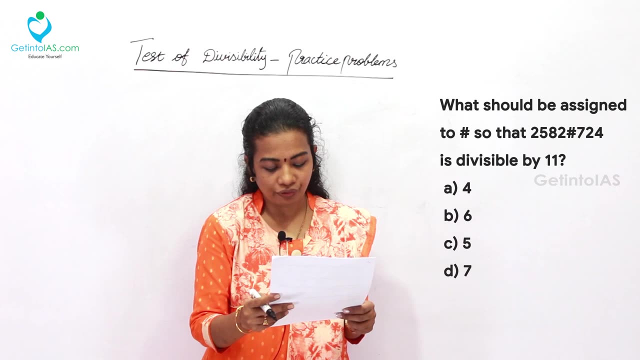 definitely a multiple of 8, and the 7 digit number is also a multiple of 8. so this number is multiplied by both 5 and 8. we can say option c is the correct answer. then the next question: what should be assigned to hash so that 2582 hash 724 is divisible by 11? 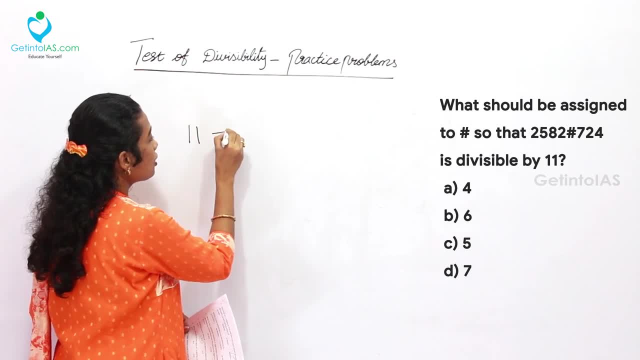 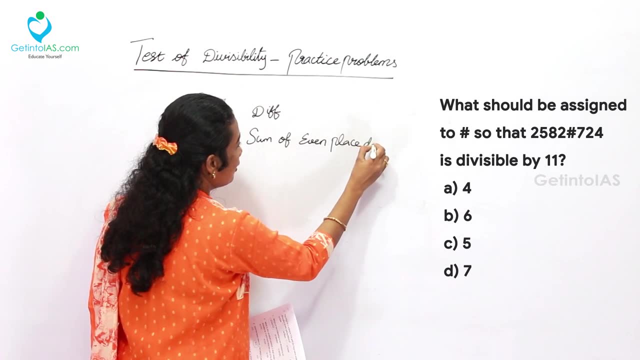 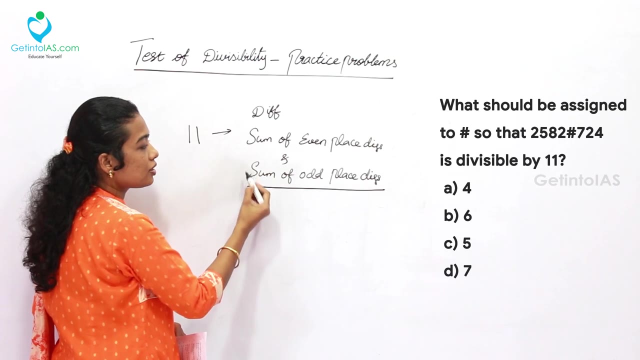 what is the rule for 11? divisibility rule for 11 says the difference between the sum of even place digits and the sum of odd place digits. the difference between the sum of even place digits and the sum of odd place digits should be the same. so the difference between the sum of even 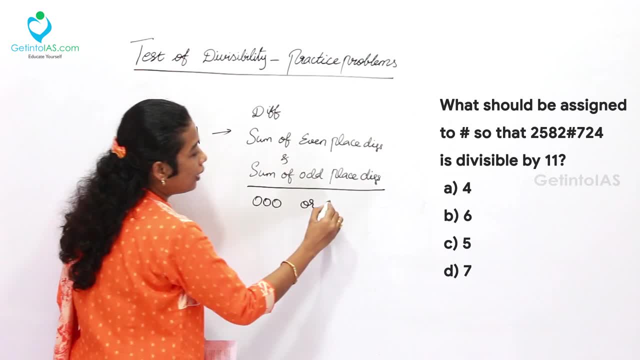 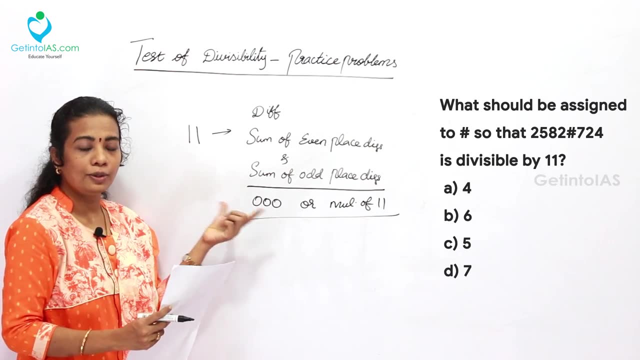 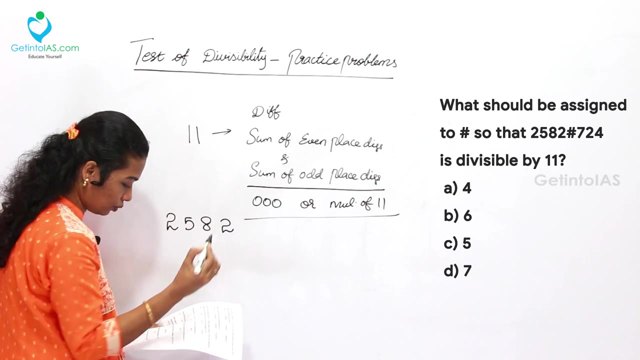 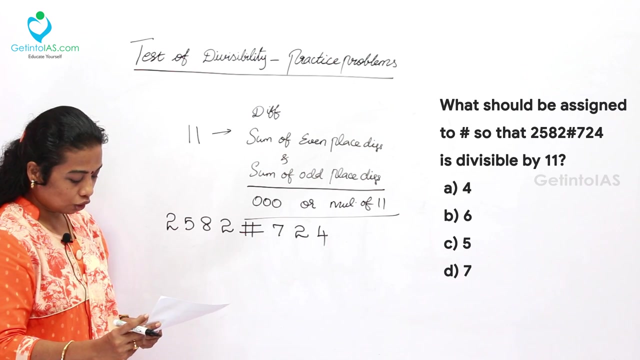 place digits and the sum of odd place digits should be 0 or a multiple of 11. so which number is satisfying these conditions will definitely divisible by 11. looking at the number which is given: 2582 hash 724. this is the number given here. the 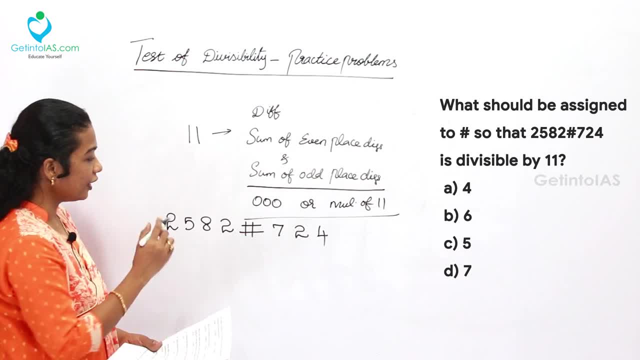 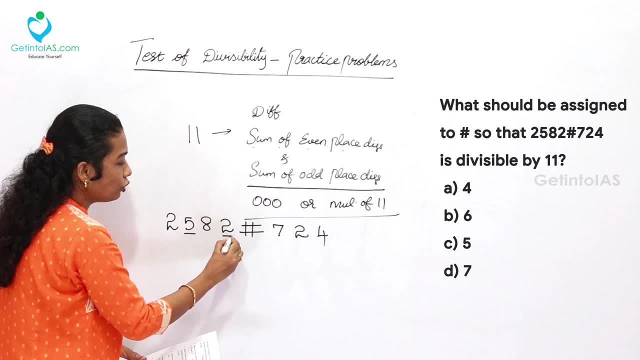 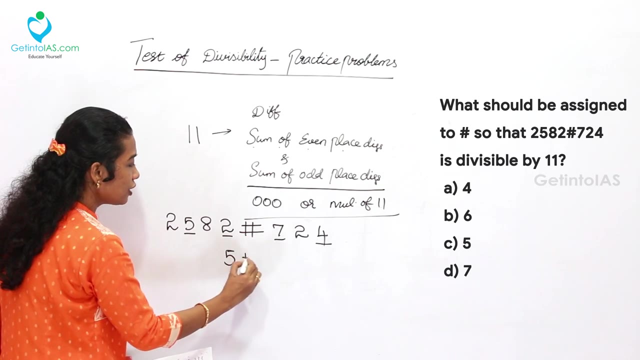 options are saying 4, 6, 5 and 7. so let us take the sum of even place digits first. even place means second place, fourth place, sixth place and the eighth place. so adding 5 plus 2 plus 7 plus 4, so what is the result? 5. 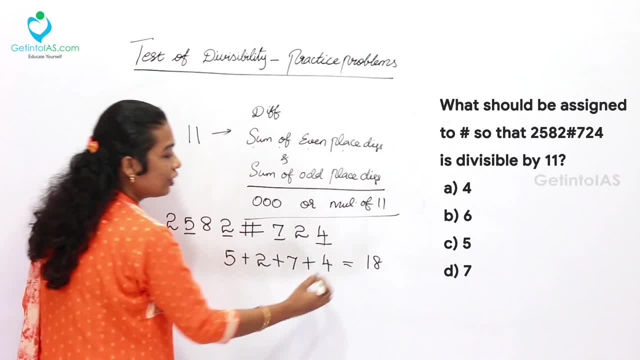 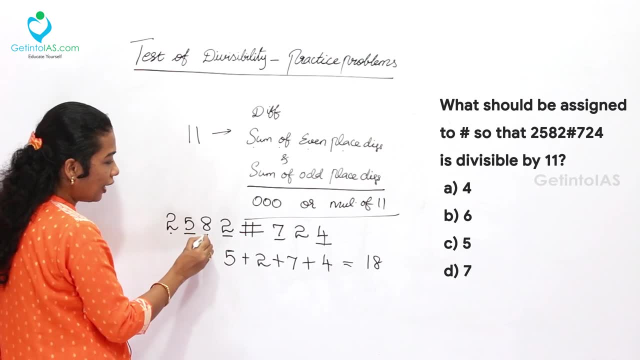 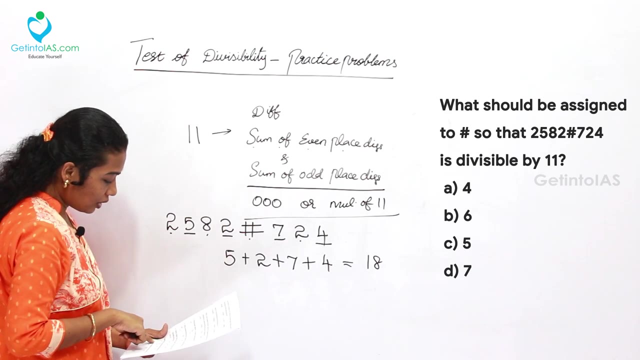 plus 2, 7 plus 7, 14, 14 plus 4, 18. I got the even place digits here. then the next one: odd places. what are the odd places I am making dot over here? 2, 8 hash, and the second place is 6 and 2 hash. we don't know the value at present, but options are. 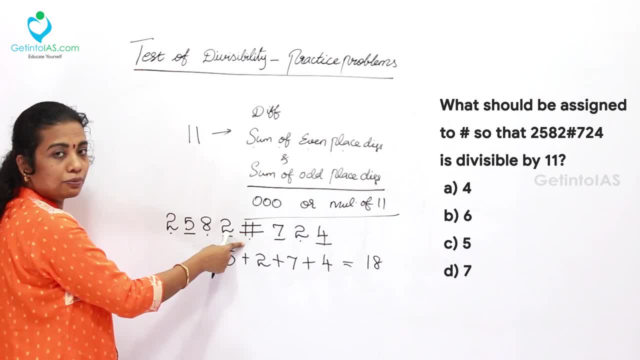 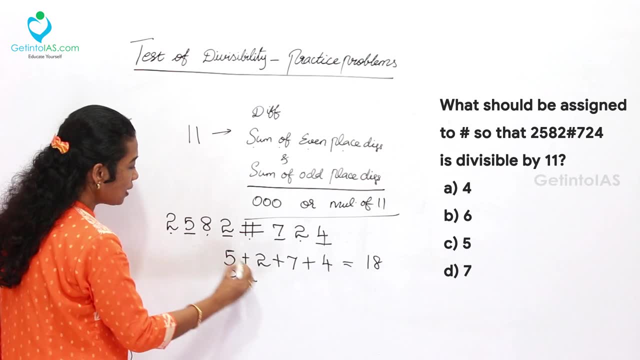 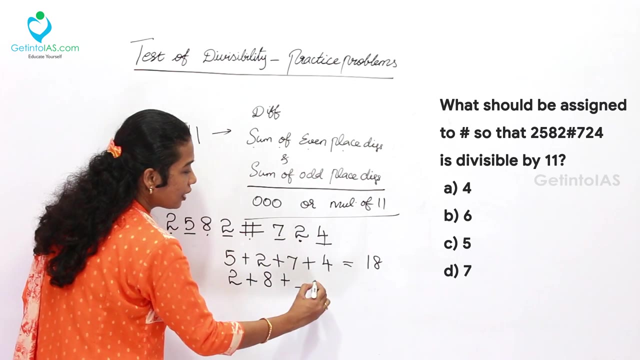 given 4 values: option a: 4, 6, 5, 7, 1 by 1. we are going to substitute instead of the hash symbol. so let us take first: 2 is the odd number plus 8, then plus leave for the hash symbol, then you can take. 2 is the next number. now let us substitute. 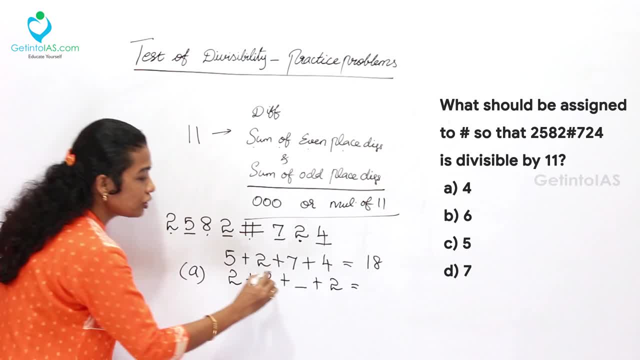 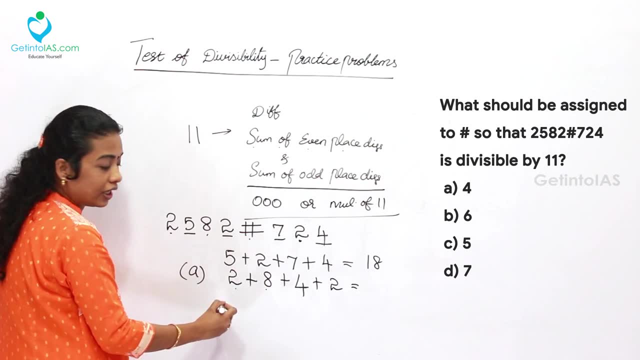 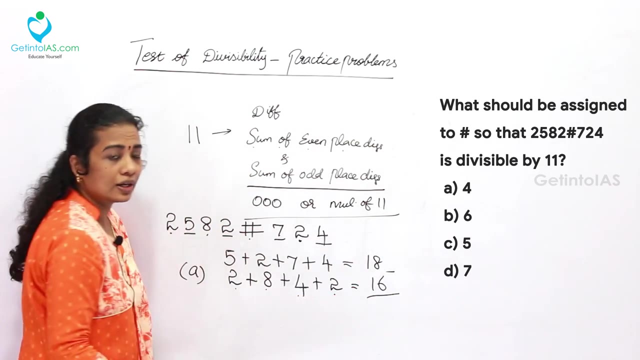 here. option a: what is the value given, which is 4? so simply, I am taking 4 instead of the hash value. now you can add up 2 plus 8, 10, 10 plus 4, 14 plus 2, 16. now test for the difference. that is 18 minus 16. the result is 2, which is not. 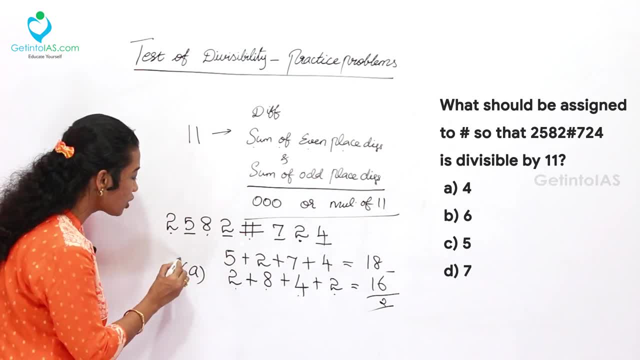 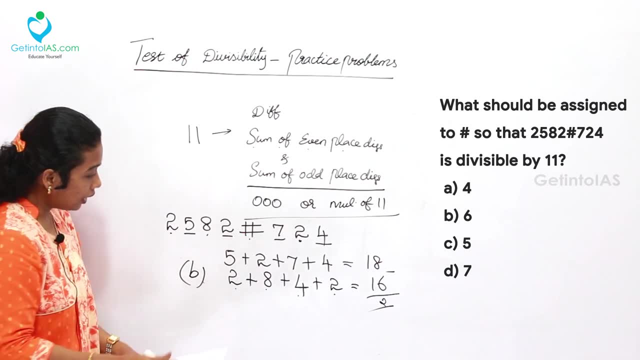 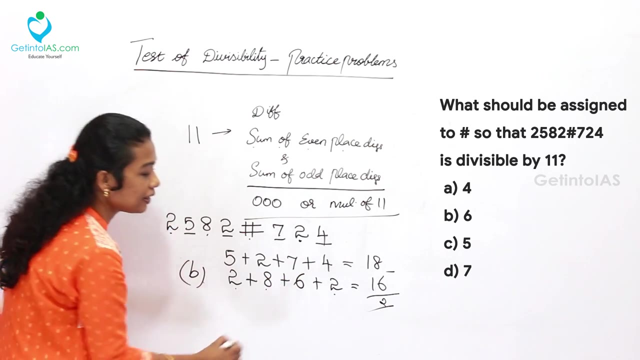 equal to 0 or a multiple of 11. so option a ruled out. let's substitute option B's value over here, option B, which is saying the hash is to be replaced by 6. so simply I am removing the option a, value 4, and making 6 here. then the sum will. 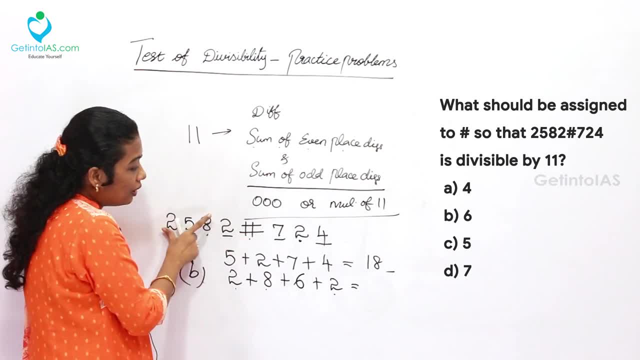 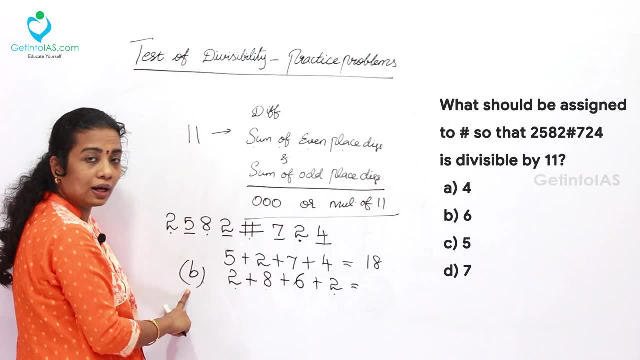 get changed already. the even places doesn't have any change, so this sum will not get changed. the second line, odd places, will definitely get changed. why? because we have taken option B's value over here. so 2 plus 8, 10 plus 6, 16, 16. 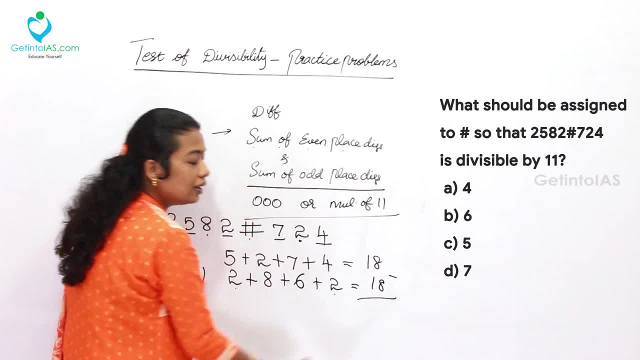 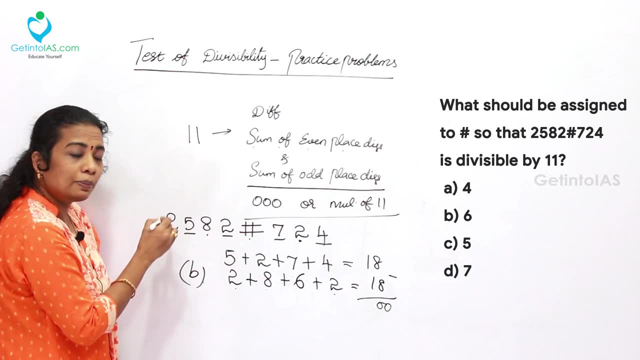 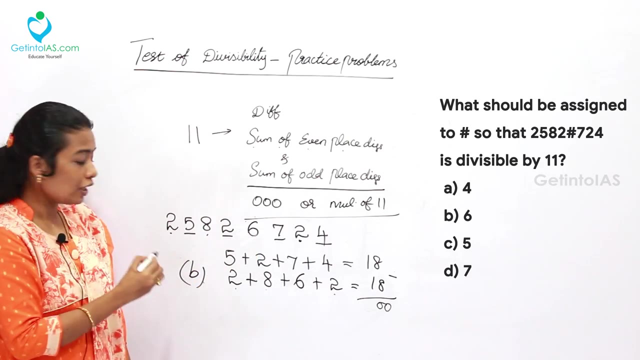 plus 2, which is 18. now you can take the difference between these two values: 0 s one of the conditions satisfied. so this number is definitely divisible by 11. what number? 2, 5, 8, 2 and 6, 7, 2, 4. this number is divisible by 11, so the option B is the. 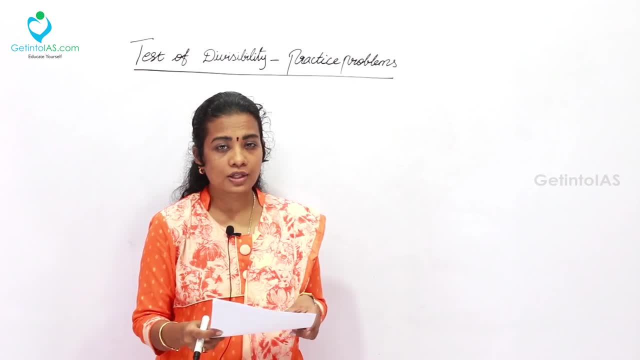 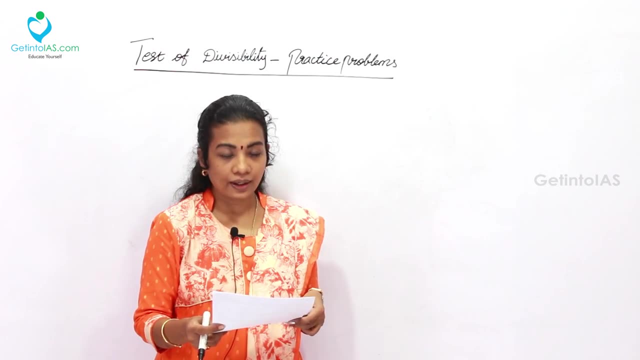 correct answer. as of now, we have solved the problems by using directly the test of divisibility rule. what we have learnt in the previous session from 1 to 20 to 90, for that we didn't learn the test of divisibility rule also, it is not. 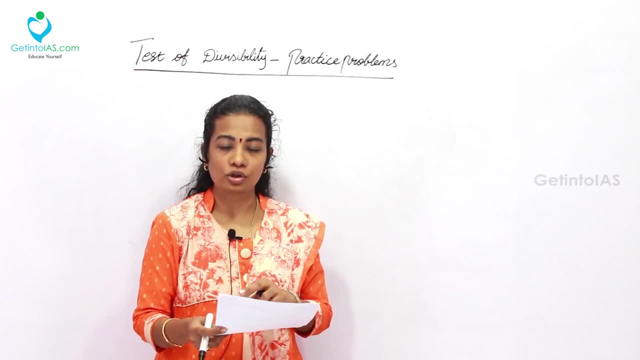 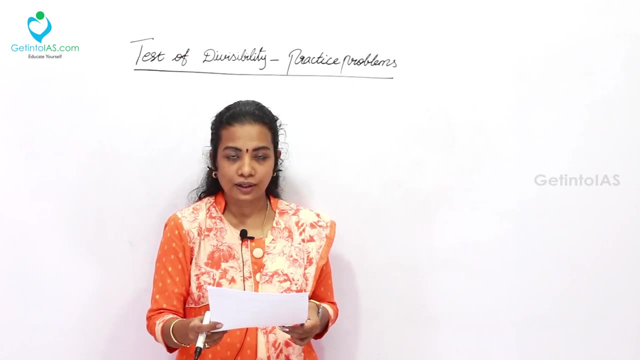 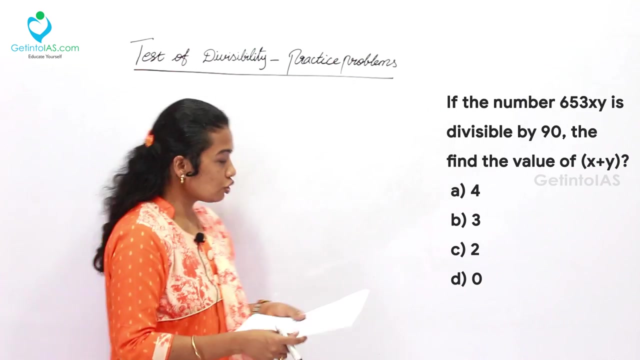 possible to learn all the numbers divisibility rules so we can make the break up for 90 as 9 and 10. the question in front of you is: if the number 6, 5, 3, X, Y is divisible by 90, find the value of X plus 5. so here a number which is a. 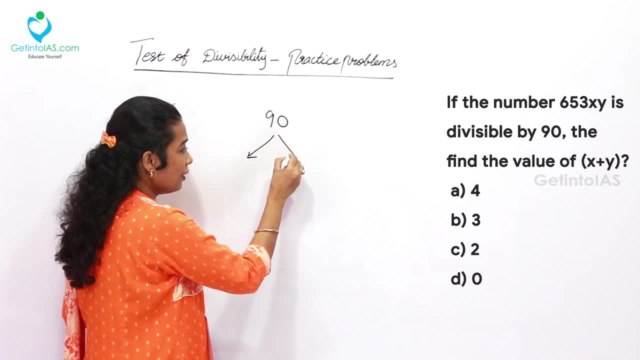 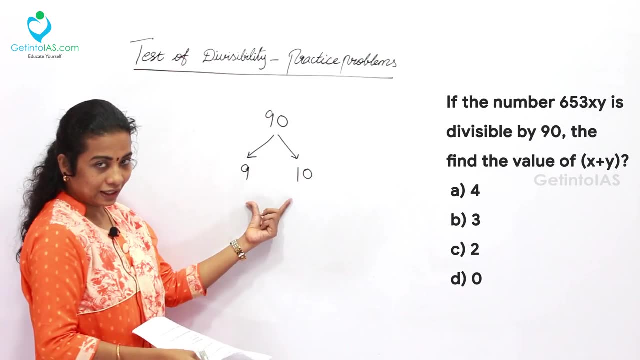 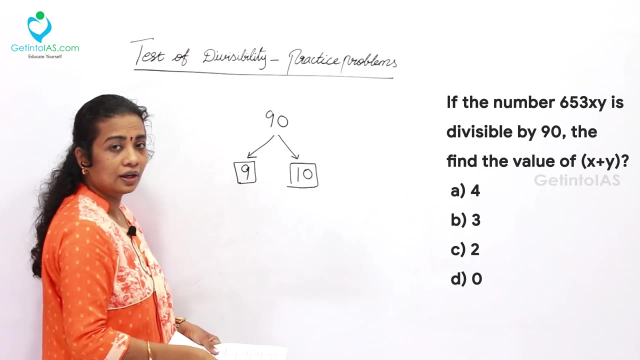 multiple of 90 should be 0, a multiple of 9 and also should be the multiple of 10 separately. so you can test the divisibility rule for 9 and 10 together and check whether this number is divisible by 90 or not. why we have taken 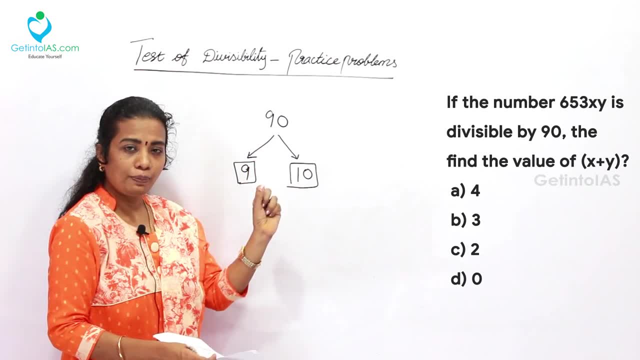 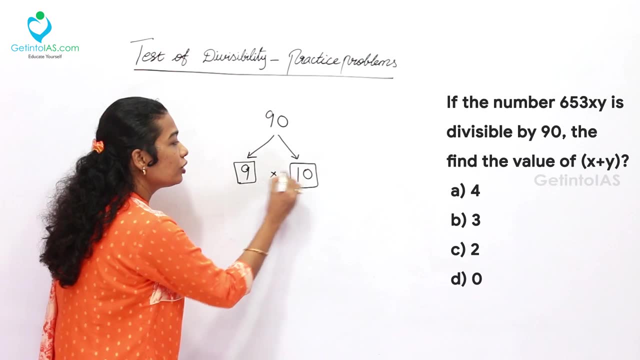 9 and 10. why should not we take 2 and 45? why? because 1 to 20 the divisibility rule is compulsory and 9 and 10 are lying within the range. so 9 into 10 is 90, simply. so instead of taking 90, you can. 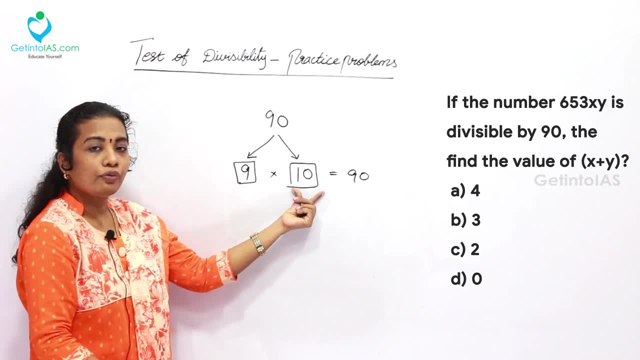 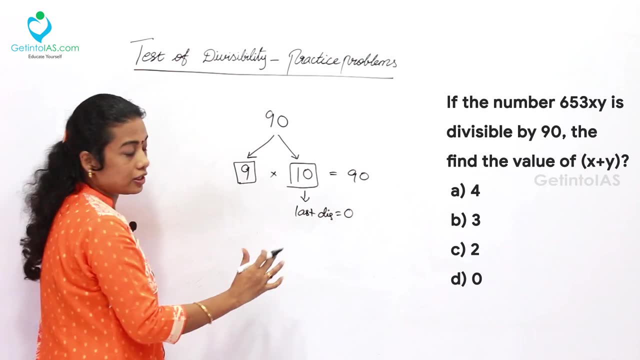 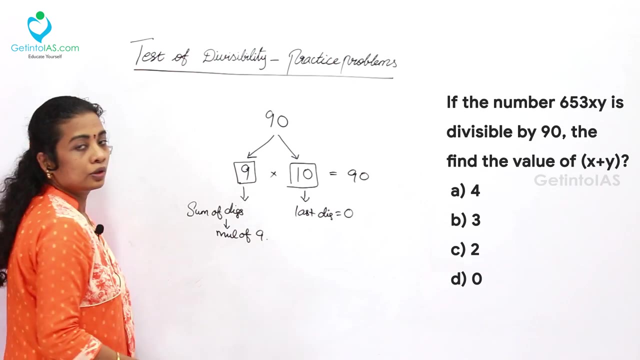 choose the test of divisibility rule for 9 and for 10. okay, what is the test of divisibility rule for 10? the last digit should be 0, always. what is the rule for 9? some of the digits should be a multiple of 9. so when these two conditions are satisfied with the number, definitely that number will be. 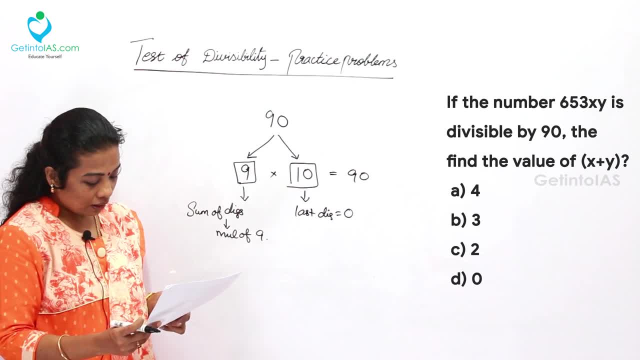 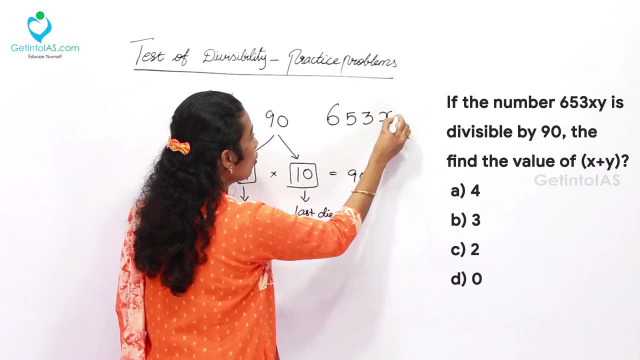 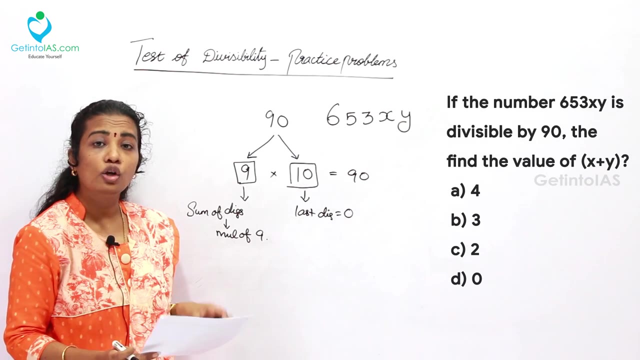 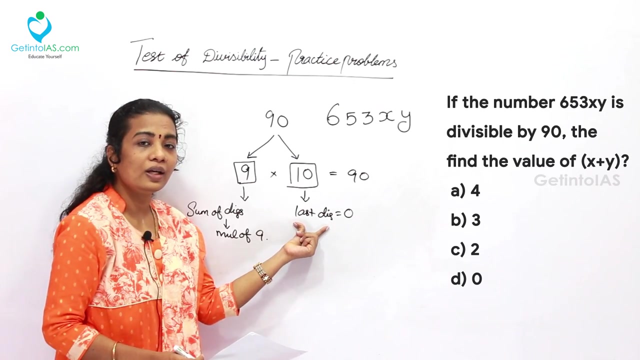 a multiple of 90. so it is given 653 x y. i'm taking 653 x- y. so your x and y are to be replaced by the numbers in the option. x and y- separate values are not given. sum of x plus y is given. okay, let us check with the easiest option. what is the easiest divisibility rule among these two? 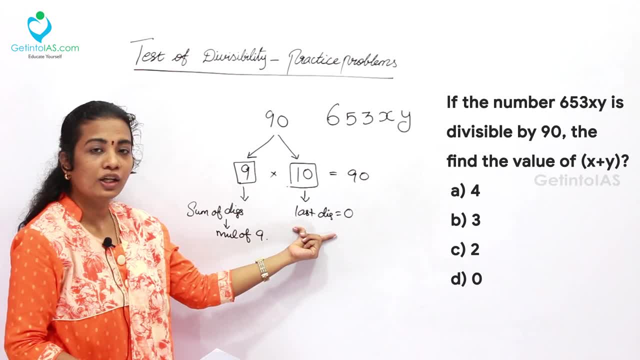 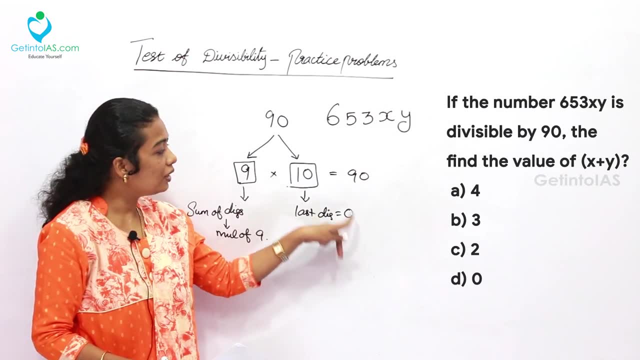 here 10, 1 to 10.. whether that number is divisible by 10 or not, how the last number should be 0, then it is divisible by 10. if it is not 0, it is not going to be the multiple of 10. so here we can say: 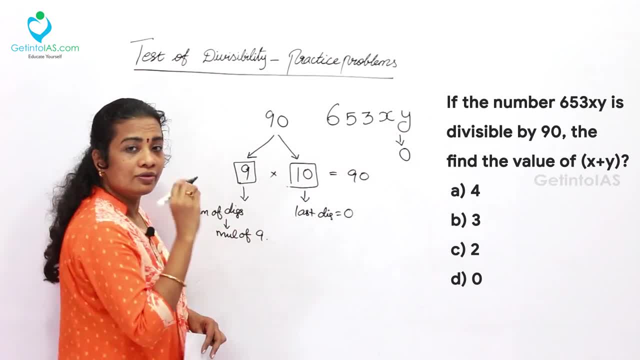 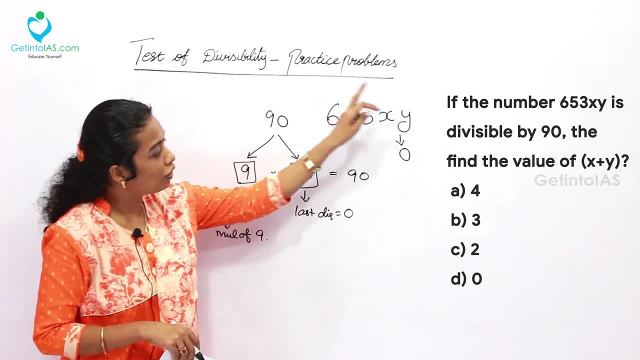 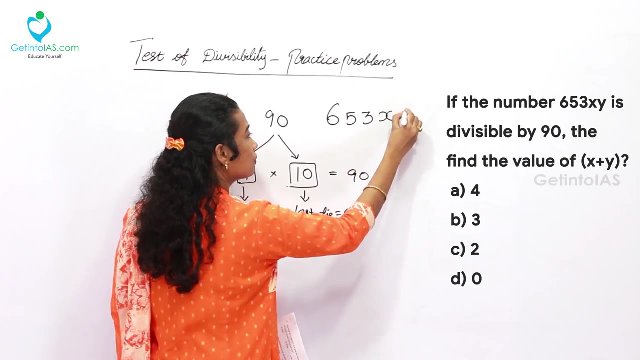 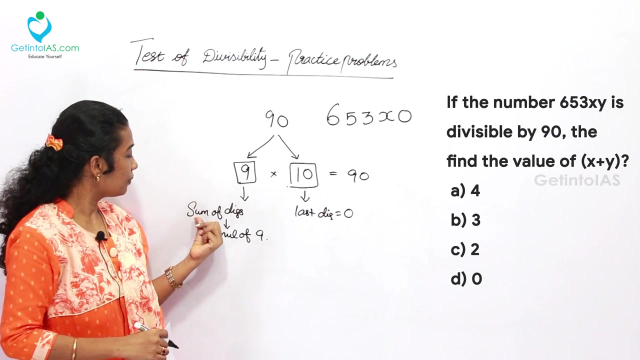 definitely y should possess the value of 0, because, it is clearly said in the question, this number is exactly divisible by 10. so as of now you got this point, you can simply go to the next step. That is, I am making here 0.. Here, 653 x 0.. Now, moving on to the next step, The sum of 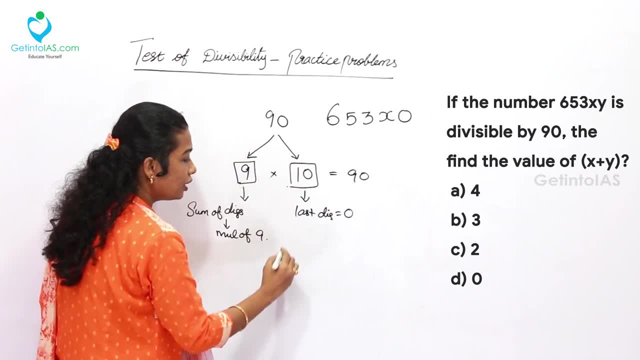 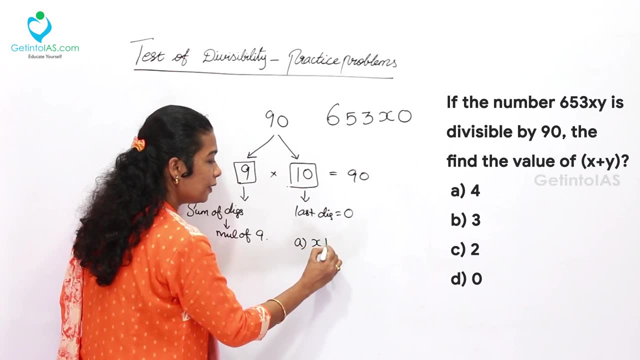 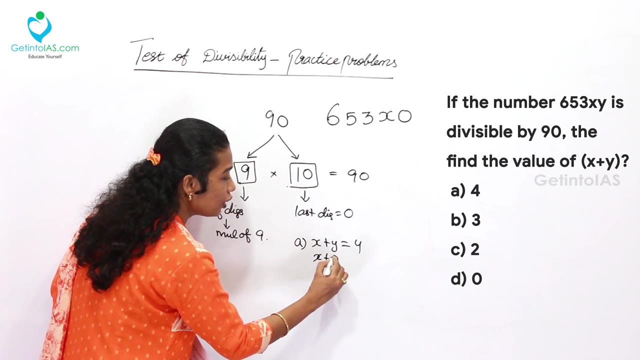 digits should be a multiple of 9.. Now you can choose with the option, Option a, which is given 4.. x plus y is 4. It is saying already we know that y is 0. So x plus 0 is equal to 4. Then x. 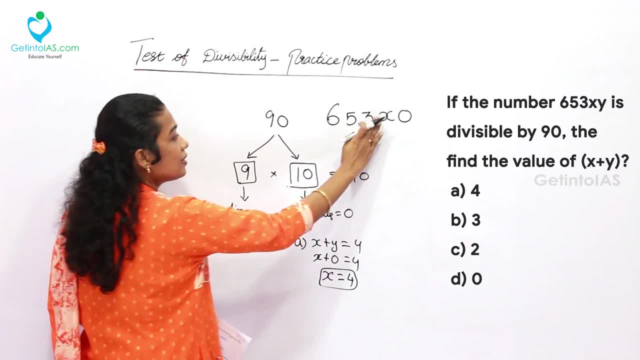 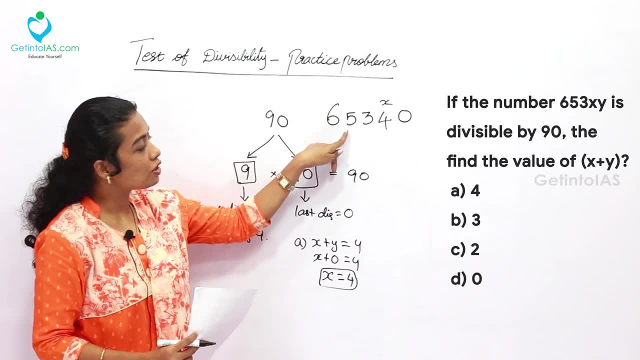 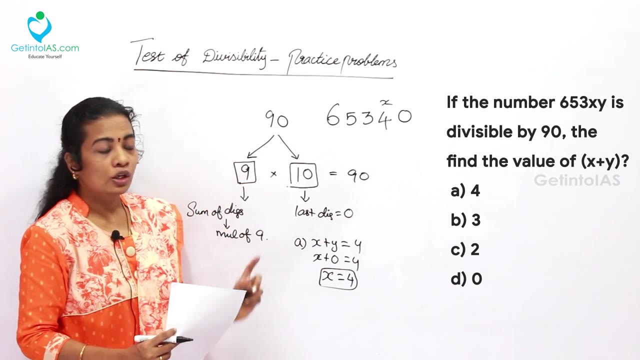 will be 4.. It is saying: So now, let us replace x value as 4.. This is x. right Now just add up all the values: 6 plus 5, 11,, 11 plus 3,, 14,, 14 plus 4, which is going to be 18.. So 18. 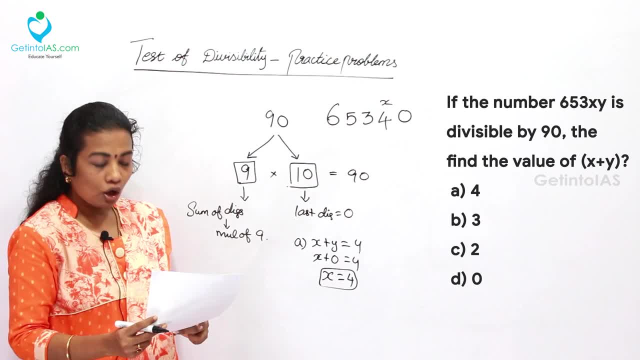 is equal to 4.. Now let us replace x value as 4.. This is x, right? Now just add up all the values 9.. So the answer for this question is option a, 4.. The next question which is similar to the: 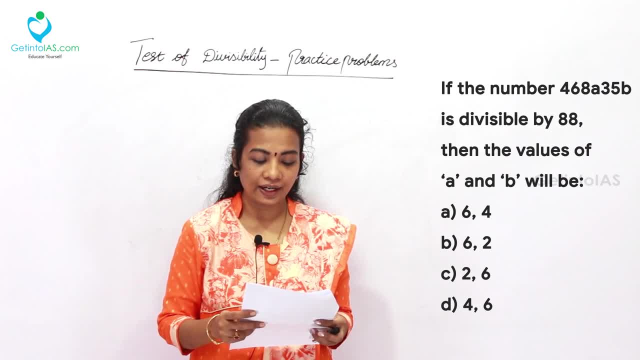 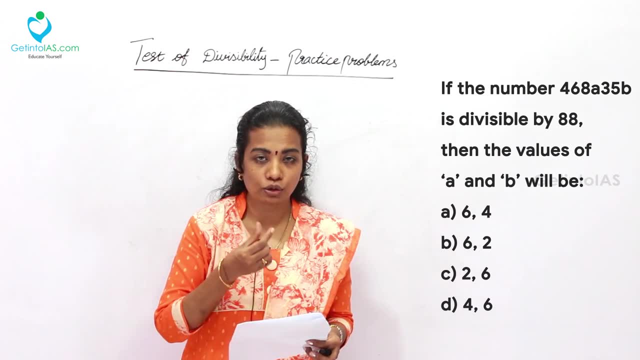 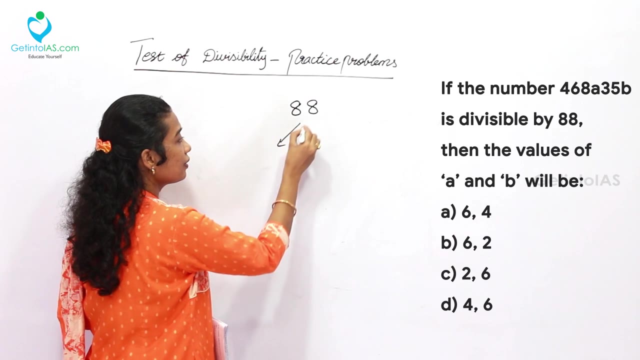 previous one. If the number 468, a35b is divisible by 88, then the values of a and b will be Here. the direct values of a and b is given and it is divisible by 88. So breakup of 88. it can be written. 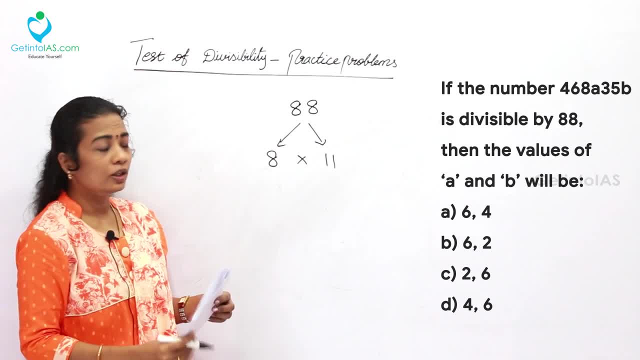 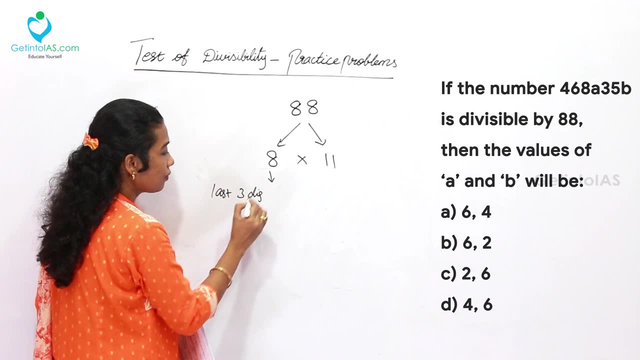 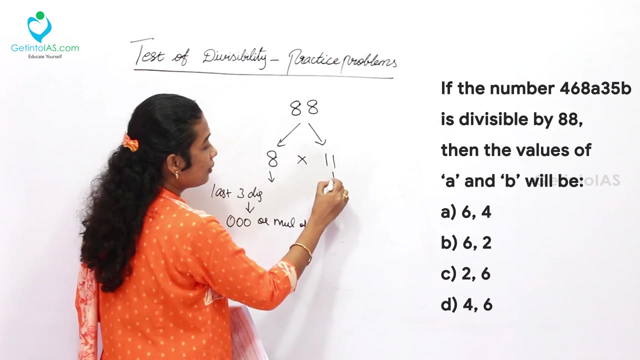 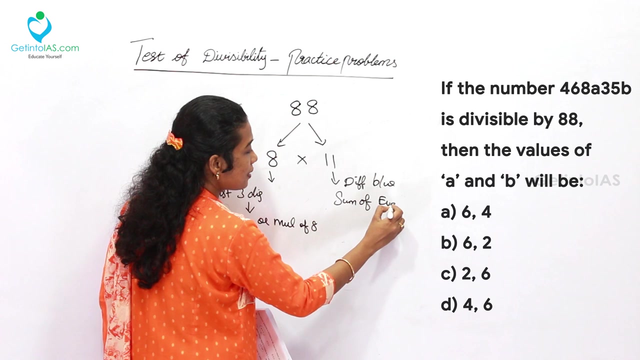 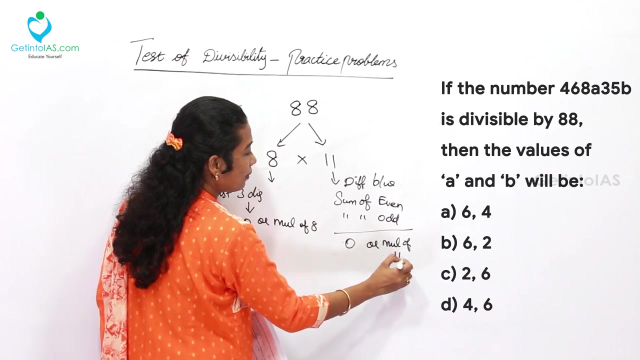 8 into 11.. We know the divisibility rule for 8 and 11.. What is the rule for 8?? The last three digits should be 0 or a multiple of 8.. For 11, the difference between the sum of even places and the sum of odd places should be 0 or multiple of 11.. 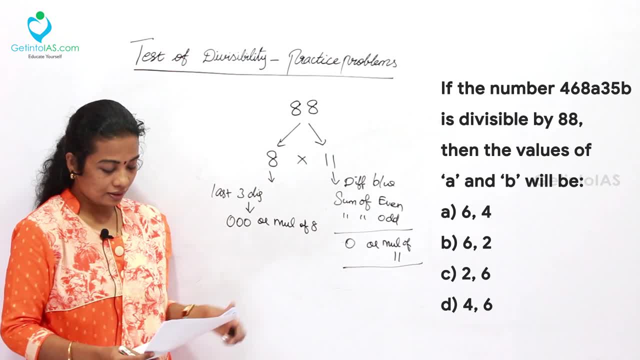 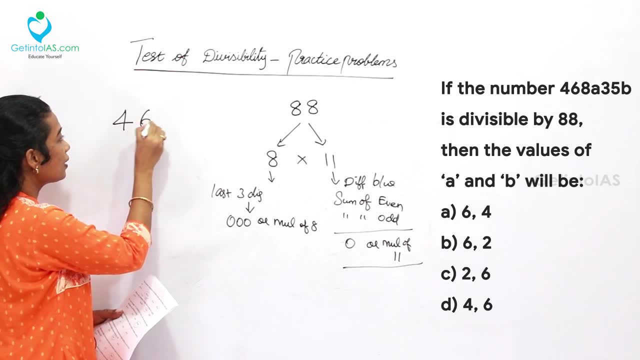 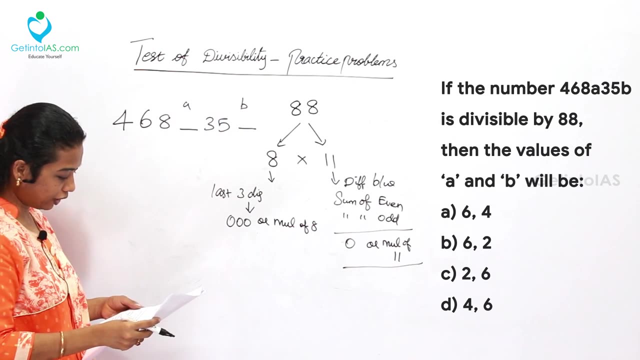 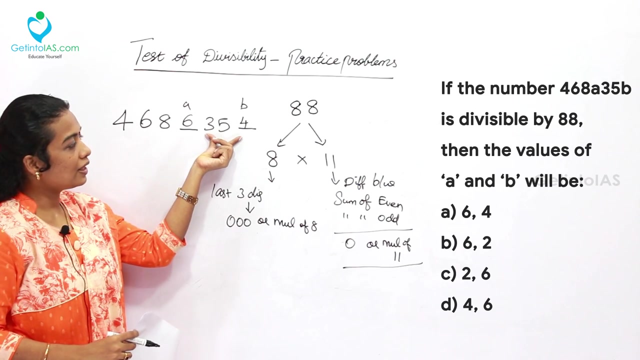 So, applying these two rules, you can easily find the answer. option a, which is given, 6 and 4.. Let me write the number, which is 468, a35b here. Here we are going to place the values one by one: Option a, 6 and 4.. Let me take 6 here, 4 here. So first I have placed. 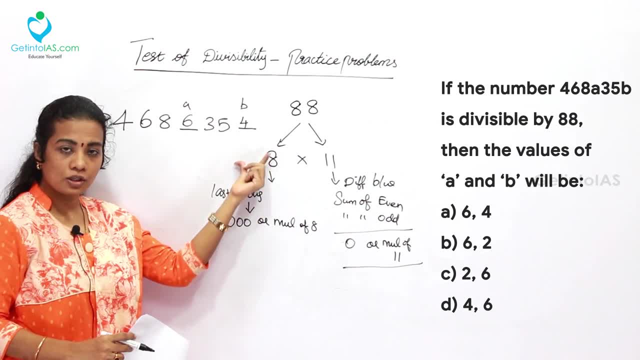 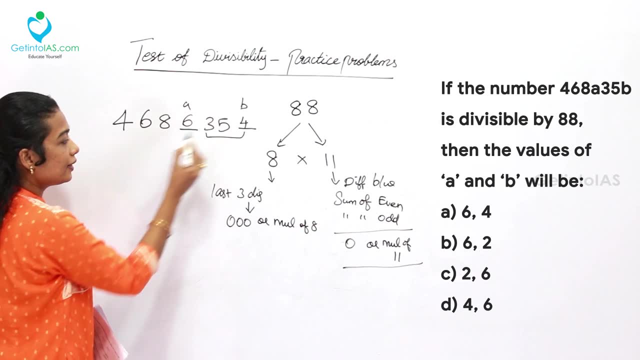 4. here First I can check with the divisibility rule with 8.. That is last three digit should be a 0 or a multiple of 8.. Here 354. let us check 354. quotient is not required here. So 8, we know 32 is a multiple of 8.. So 5 minus 2 is 3.. 34 is the. 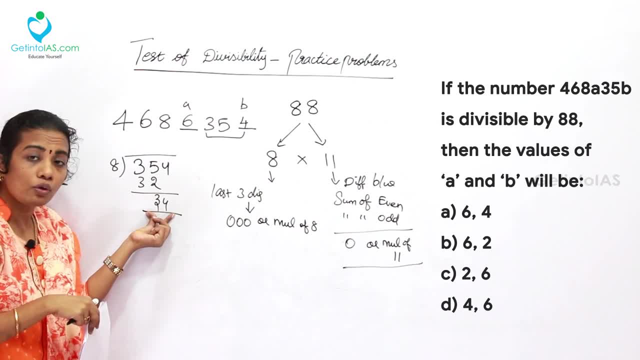 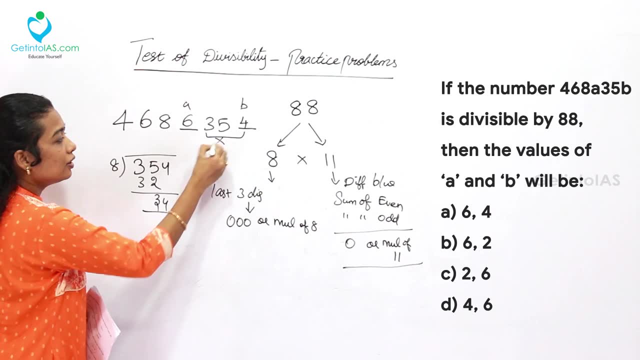 remainder. No need to do the usual division 34, just check whether it is a multiple of 8 or not. No, it is not a multiple of 8.. Only 32 is the multiple. So we can say this one is wrong If 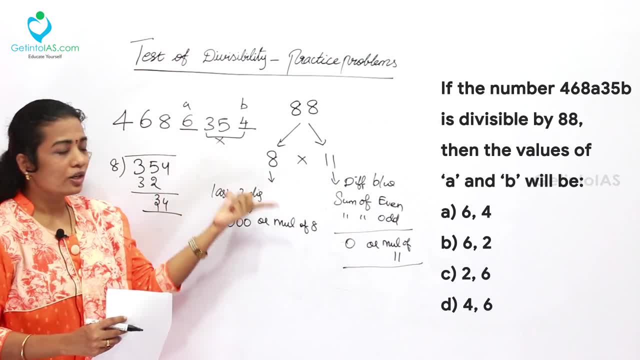 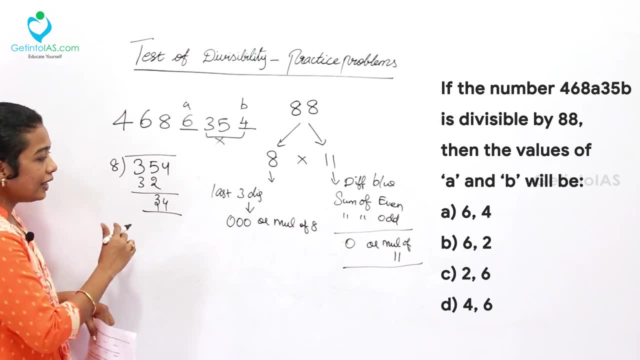 this checking, while with 11, if it is going to be the correct, what is the use? because 88, both the conditions are to be satisfied. From the point of checking with the 8 itself, I can skip. option a is ruled out. Why? because the option a value does not meet the satisfied. 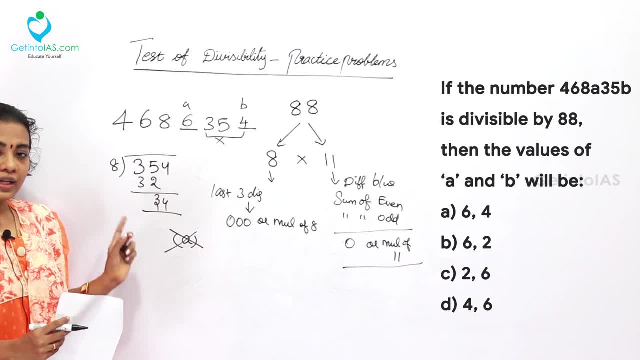 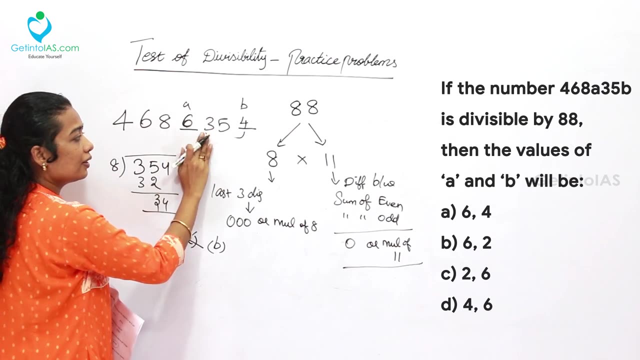 point of number with 8.. So we can easily skip it. and moving on to the option b, What is the option b says and 2, so let me take option b. a is 6, already it is here, and for b, i am going to rub the 4 and i. 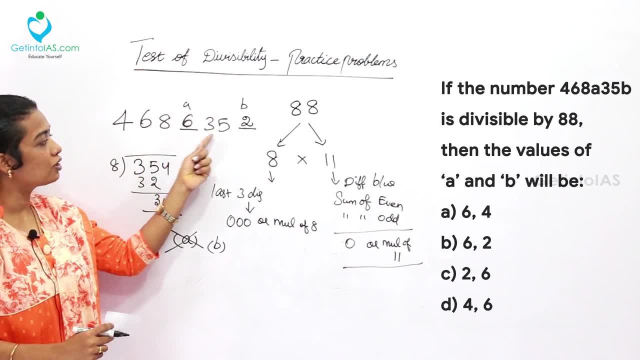 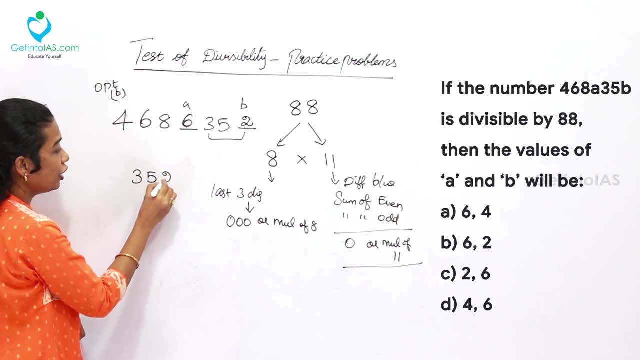 am going to write 2 now. the number required number is 4, 6, 8, 6, 3, 5, 2, so let me check with 8. so here take the last three digits: 352 while dividing by 8, so 32 is a multiple of 8. so 35 minus 32. 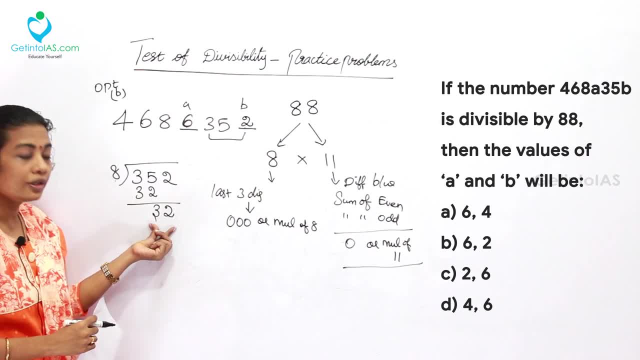 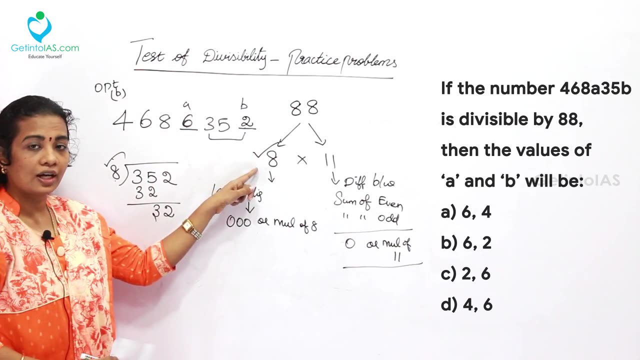 the remainder is 3, again 2 i have taken. so this 32 is again a multiple of 38, and we can say 352 is a multiple of 8. so this complete seven digit number is also a multiple of 8. first condition satisfied: if the first condition satisfied, you can move on to the next condition. 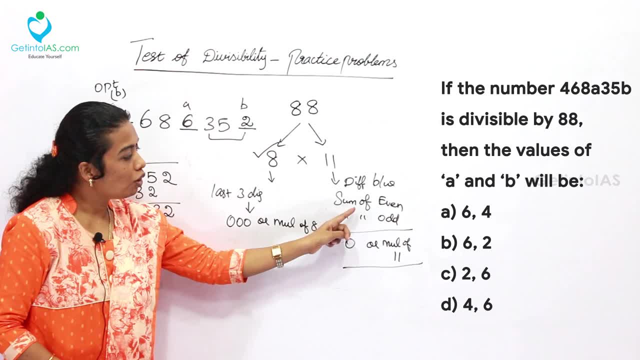 that is what is the rule for 11. difference between sum of even digits and sum of odd digits should be 0 or multiple of 11. let's do that. so what are the even digits? and some of odd digits should be 0 or multiple of 11. let's do that. so what are the? 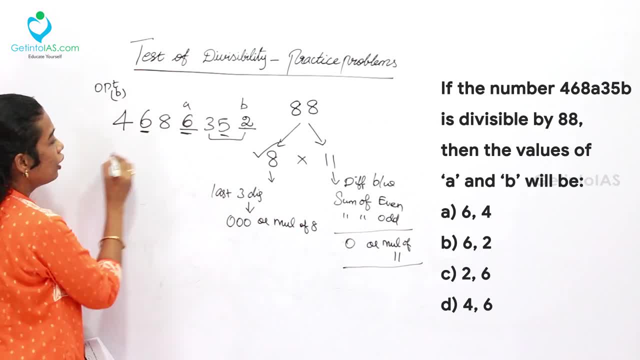 even places 6 here here, 6 here, 5, so 6 plus 6 plus 5, which is 12 plus 5, 17. now what are the odd numbers? odd places 4, 8, 3 and 2, according to option b, so 4 plus 8, 12, 4 plus 8 plus 3 plus 2. 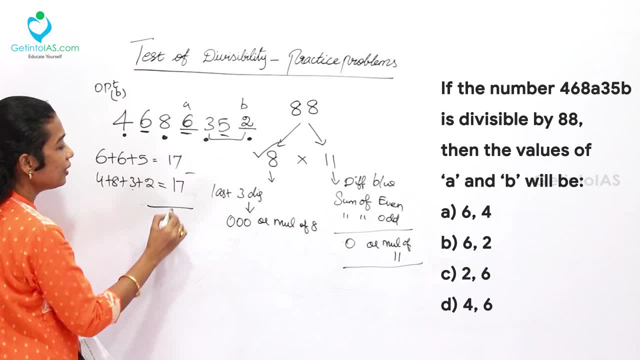 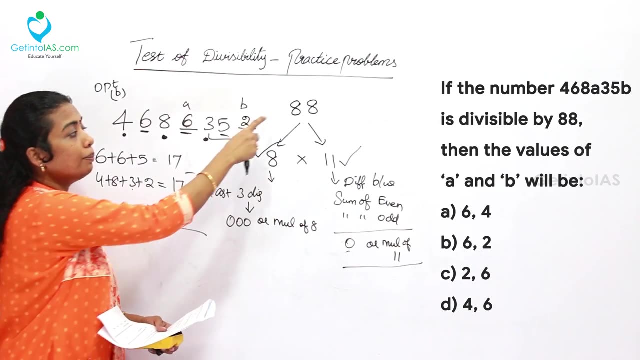 12 plus 3, 15 plus 2, 17. now, taking the difference, yes, we got 0. that is one of the condition of 11. so this number is also divisible by 11 and 8. so finally, my answer for this question is option B, 6 and 2, which is the number. 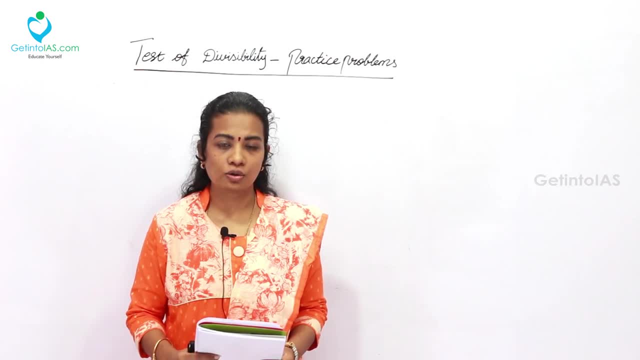 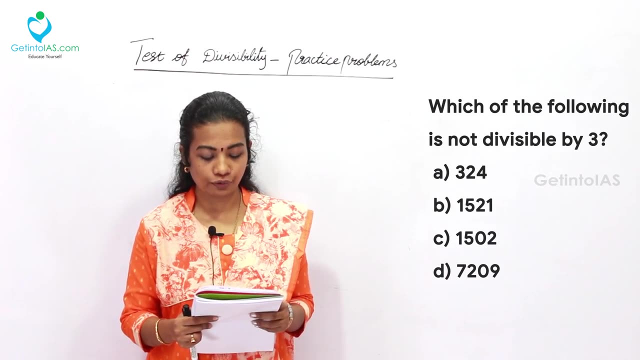 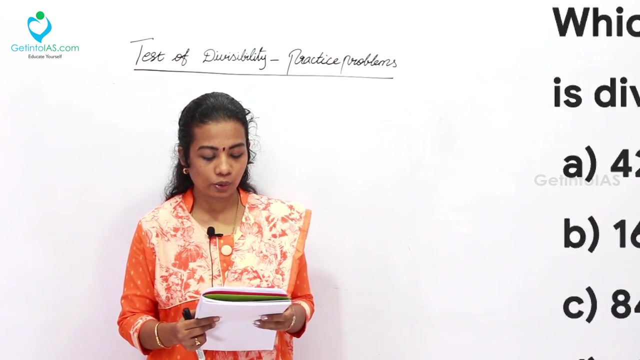 which is divisible by 80 H. now it's your turn to answer the questions. the first question: which of the following is not divisible by 3? option a: 324, option B: 1, 5, 2, 1. option C: 1 4, 0, 2 and option D: 7, 2 0, 9. the second question: 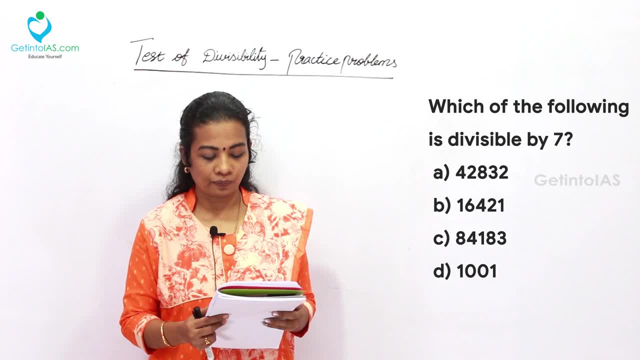 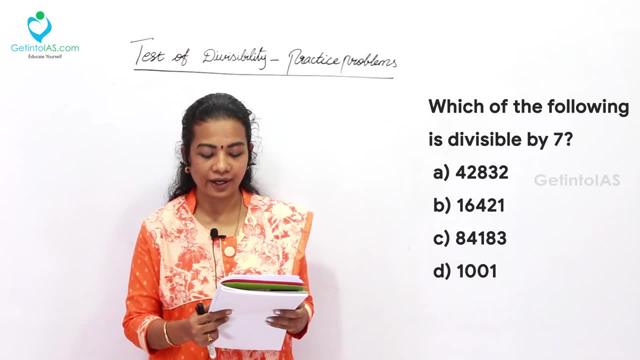 which of the following is divisible by 7: option a: 4, 2, 8, 3. 2. option B: 1, 6, 4, 2, 1. option C: 8, 4, 1, 8, 3 and. option D: 1, double 0, 1. give me your answer in the comment. 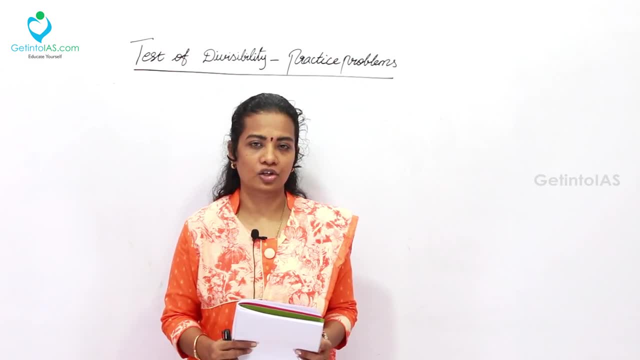 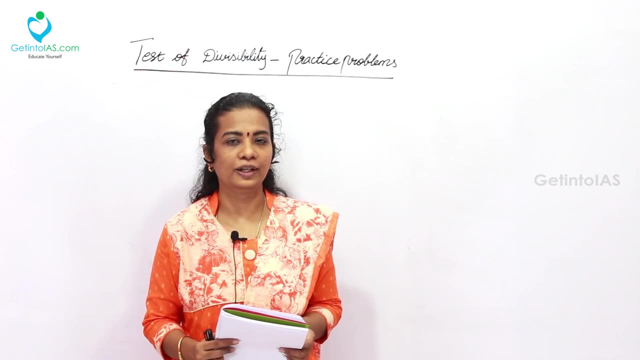 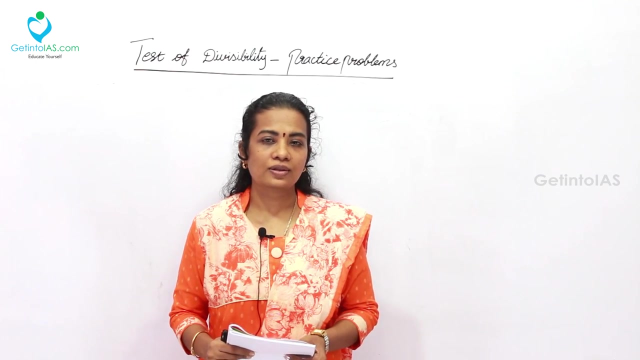 section below. subscribe our channel for more upcoming sessions. in the next video we are going to deal with some of the other kind of problems based on test of divisibility that is based on LCA method and based on the division method. you can check your answers in the description box link. follow the link to. get the answers. 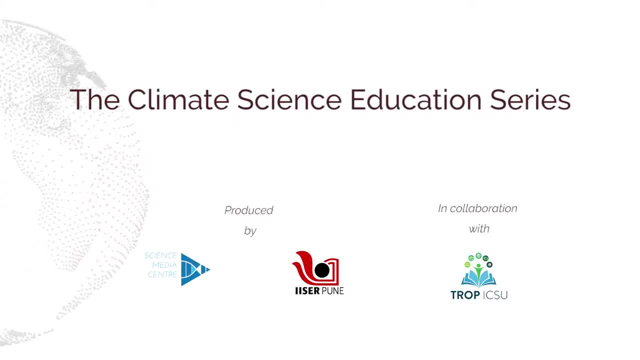 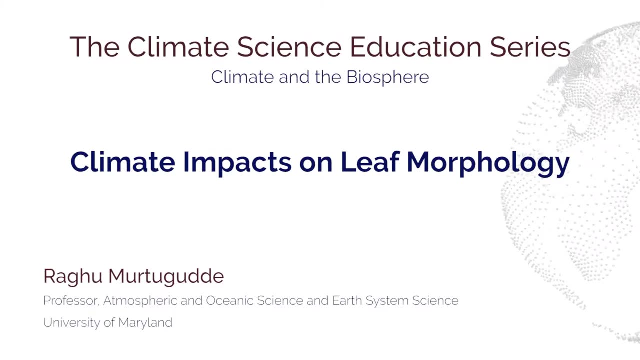 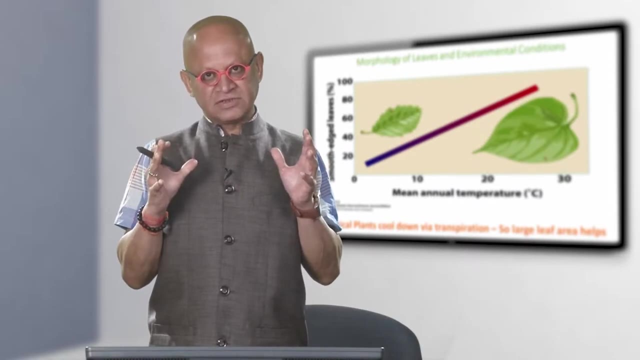 If we want to see the impact of climate on the biosphere, then we can look at very specific things. So let's look at one example where we will see the impact of the mean temperature: annual mean temperature. So if you average the temperature all days of a year, what is? 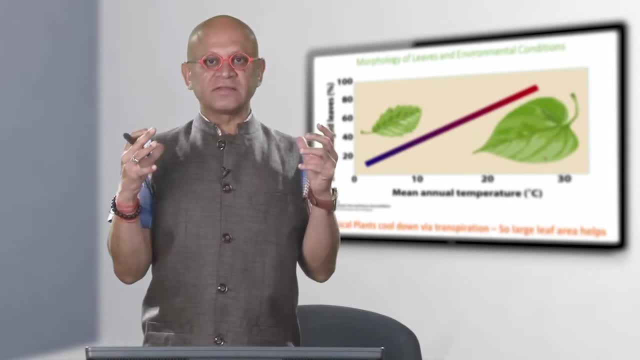 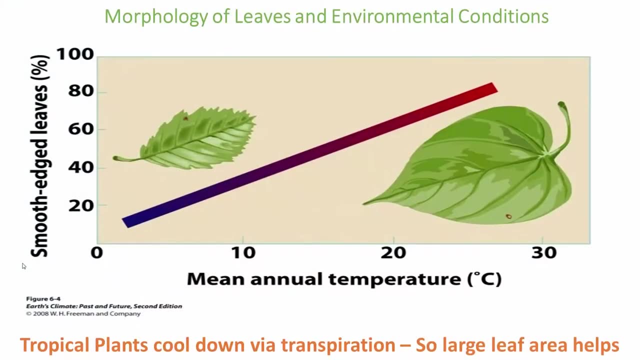 the average over a long term. How does that affect the leaf morphology, the size of the leaf, the shape of the leaf and so on? So here is an example that's showing the mean annual temperature on the horizontal axis, going from very cold temperatures at zero. 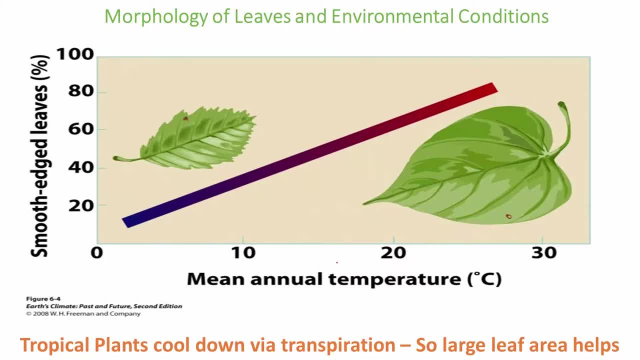 degrees centigrade to tropical temperature of 30 degrees centigrade, And on the vertical axis we have the percentage of smooth edged leaves okay. So you can clearly see that as the temperature increases there is a increase in the size of the leaf if you compare to.